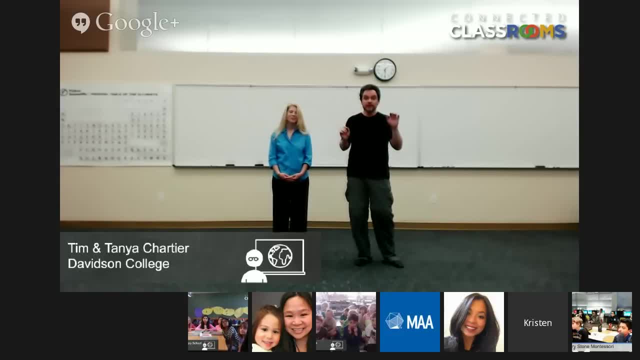 Today we're going to show you some of the mysterious things of mine- and sometimes they seem rather magical- And how they can connect to mathematical ideas that you can think about and possibly even study in your classrooms. So let's get started with an illusion that Tanya can teach us. 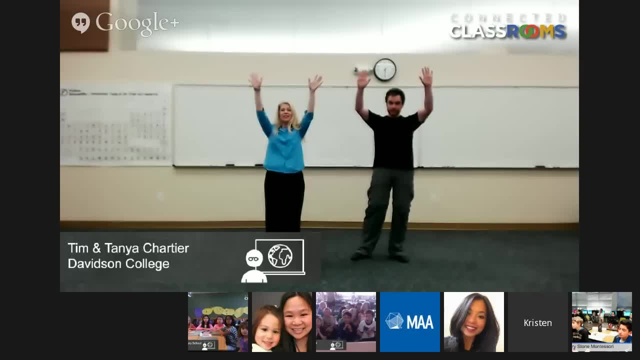 Alright, let's learn to do that together. Put your hands up in the air, Put your hands on your head. Feel that they're a little bit rounded in shape. Now take them off your head and try to keep that same shape. Good job. 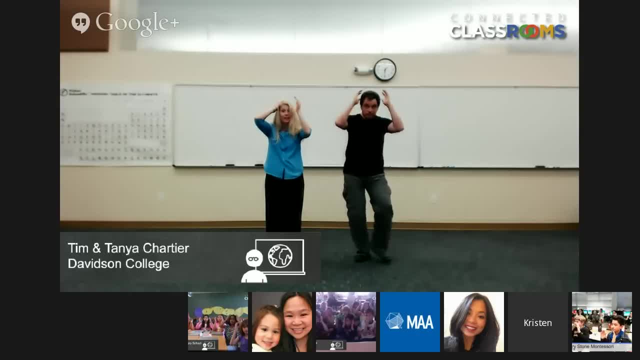 You can straighten them. and now try to go back to that rounded shape. Check, See if they're still rounded. Good, Take them off. Turn them toward me. Take one and make it flat. Take the other one and make it flat. 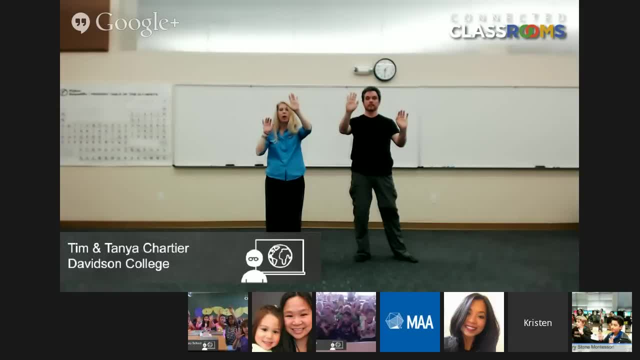 Take that first one off the wall and round it as you move it away from the wall And then put it back in a different place and make it flat. Take your second one and do the same thing. Repeat that pattern. Flat, Take one off. 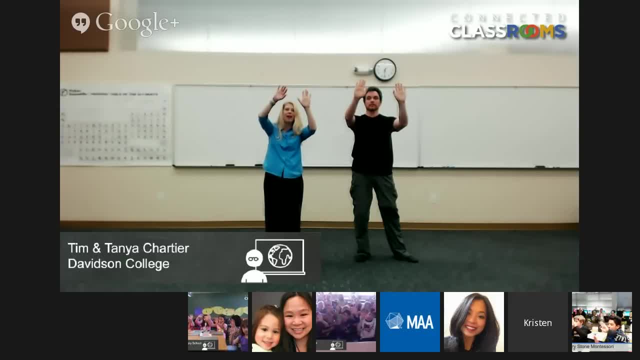 Move it, Make it flat. Take one off, Move it, Make it flat. As you continue to do this, you are creating a wall and you have to use the idea of approximation of distance and measurement, For if I went like this, suddenly the illusion is blurred. 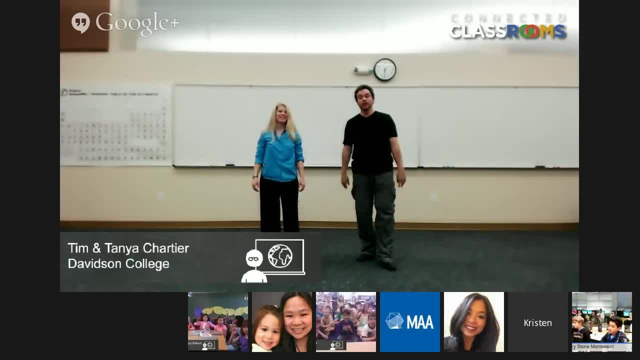 Very nice job. When you do the wall, you also use geometric thinking. When we were just doing the wall together, it was a flat wall. You can use a flat wall and then be in the proverbial mind box that people talk about. 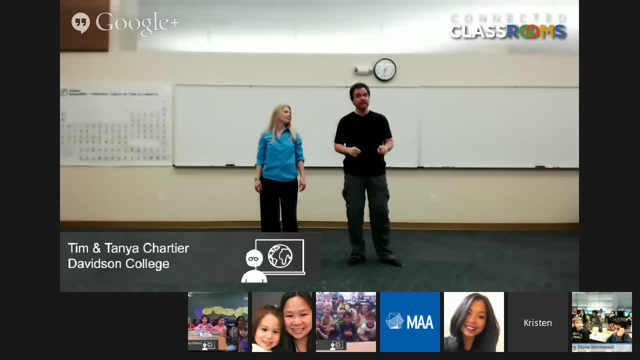 So let's try that together Now. you're in a lot of different classrooms out there, so be careful of your neighbor. So let's go up and first make your wall Remember, if you can't remember the shape when you come off the wall. 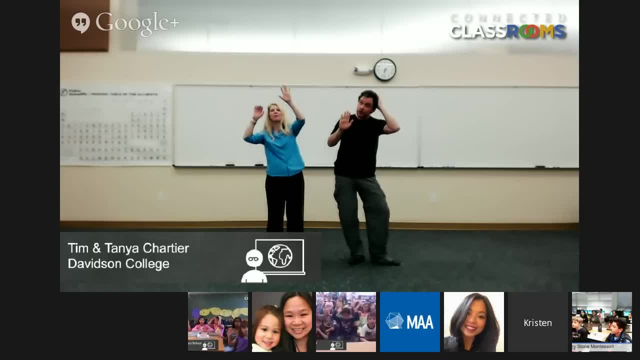 you can always check your head. If you can't check, you've got another problem going on. All right, So get it on the wall. Good, Now see if you can make a ceiling. Can you go up and get a ceiling? 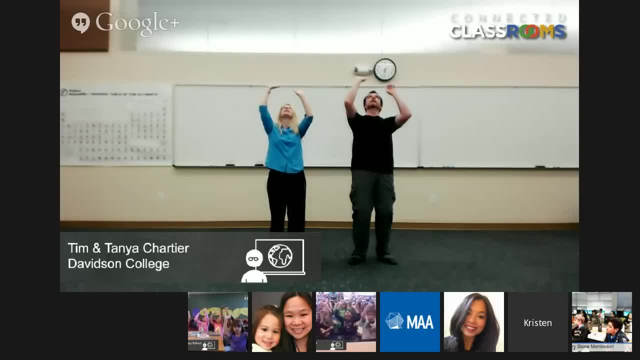 Tiny's got hers. Can you do yours? I'll make mine. How's it going? You have a slanted roof, That's okay. Got a vaulted ceiling, That's all right. There you go, Good. Now this is the one. you've got to be careful of, your neighbor. 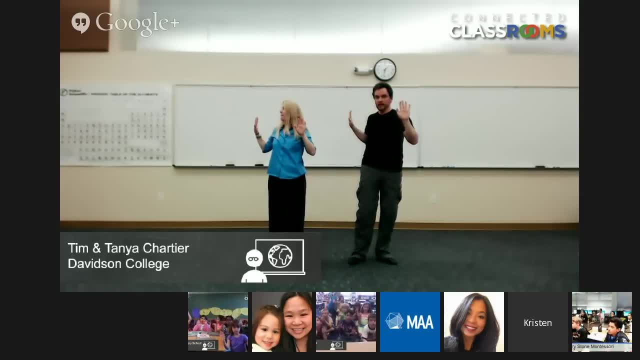 Try to make the side of the wall All right, So go to the side. Good, Now here's another one. Put yourself inside of a sphere or inside of a balloon. Can you do that? Round your hand, just like that, Round your hand. 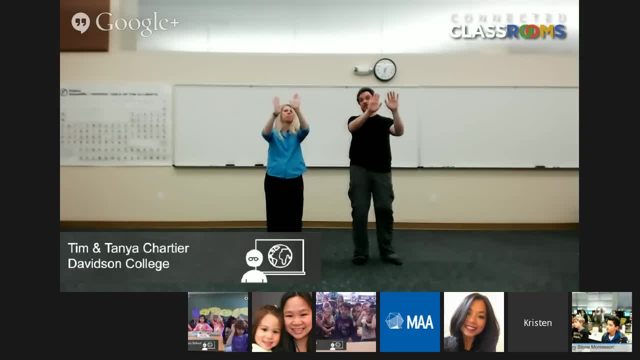 Now my hand rounds a lot. I don't know why it does that. Tanya's hand doesn't round as much, but it does round as much. Can you try See how you do with that? Good, Now there's one important thing about the wall that's very important to remember. 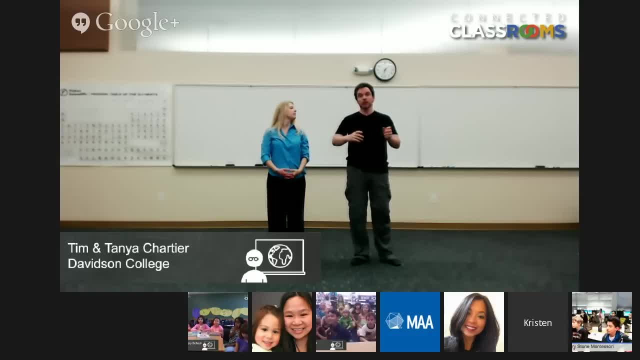 Tanya and I were very fortunate to train with Marcel Marceau, who's the world's most famous mind, when he was alive and still today, And Marceau would often say that it is not so important that you make a perfect wall. 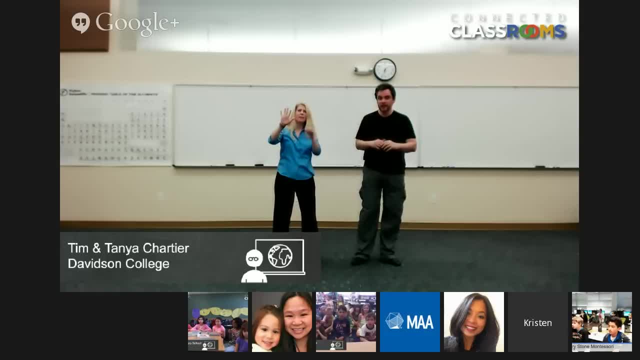 but that you make a wall for a purpose, that there's a reason that you're touching the wall. So do your best to make your hands about the same, but, as Tanya said, it's approximation, So they don't have to be exact. 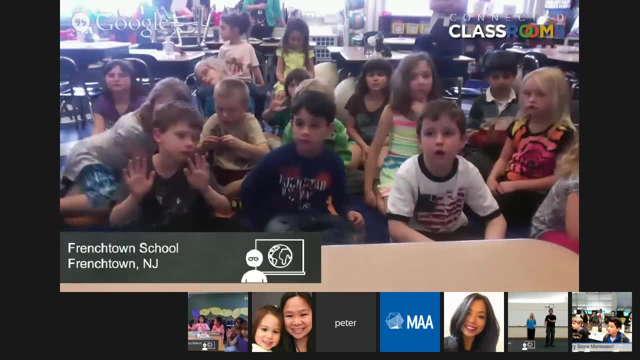 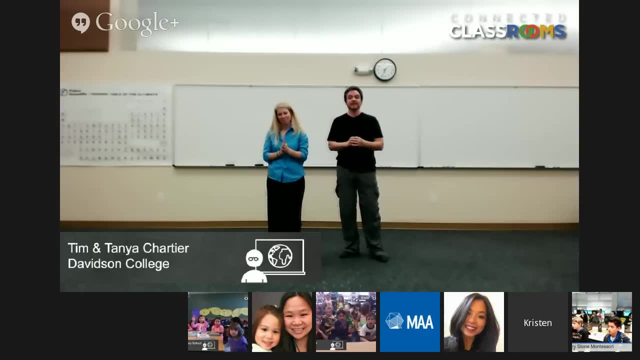 You don't have to worry that much about it, Just have a reason for what you're doing as you move along. So the first sketch that we're going to do for you will be a sketch I do on my own, and it's a sketch about the infinite infinity. 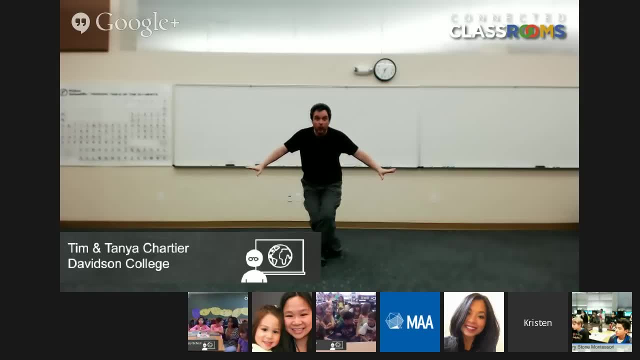 So what we're going to do is imagine that on the floor there's a rope and it goes on forever in both directions, because it's an infinite rope. So it goes on forever in this direction and on forever in this direction. So watch this sketch and watch for ideas of infinity. 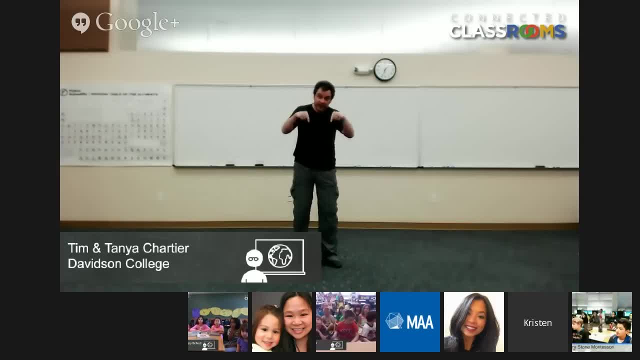 I'll ask you one at the end that I ask my students here at Davidson College in our math classes. Then there's a secondary idea that I may just refer to really quick that we use in calculus class here at Davidson College as well. So again, enjoy this sketch about the infinite rope. 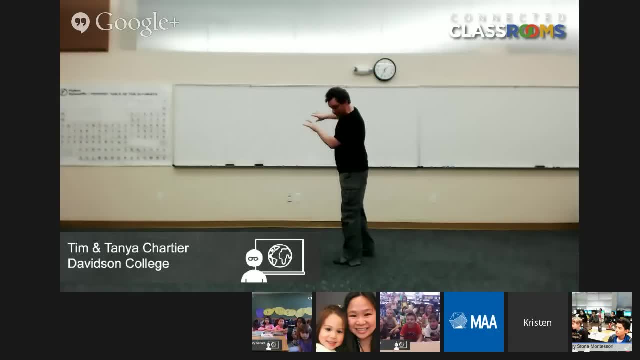 All right. And there's the infinite rope- All right. So the mathematical idea comes in the middle of the sketch, basically the middle. The mime me grabs the rope. 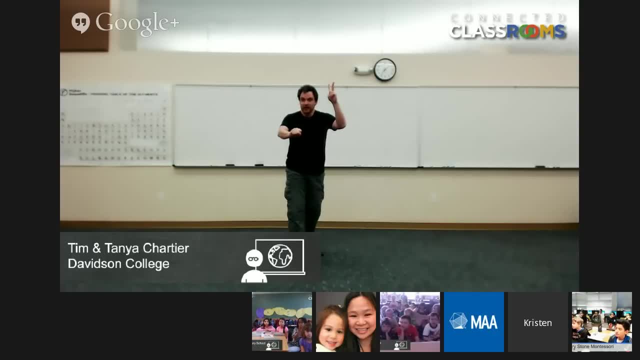 I have the rope in my hand and I bring it out And I cut the rope and a huge part of it goes away. How much rope do I still have in my hand? How much rope is still there? Well, if you think about it, how far does it still go? 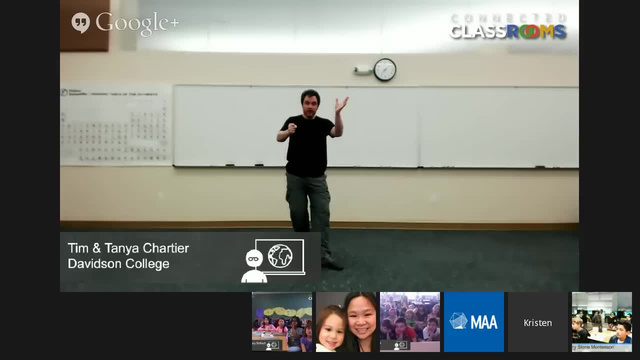 It goes on forever, So it is still an infinite-sized rope. Now, that's pretty weird. I mean anything else that we're used to, like a number four. you take part of it away and you have something else, And yet infinity is different. 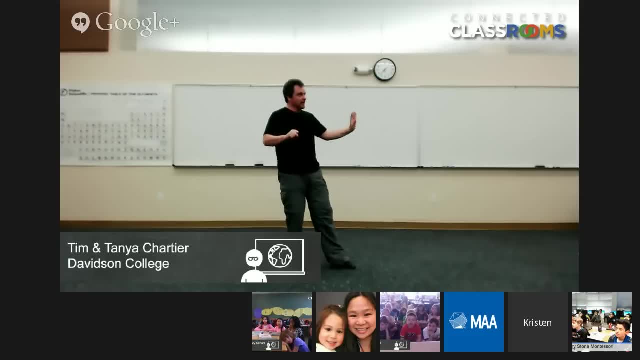 You can have an infinite amount, take away an infinite amount and still have an infinite amount. That's what I love about math: It lets us study ideas that, at one level, are so unintuitive and, at another level, let us study it in a way that we can understand. 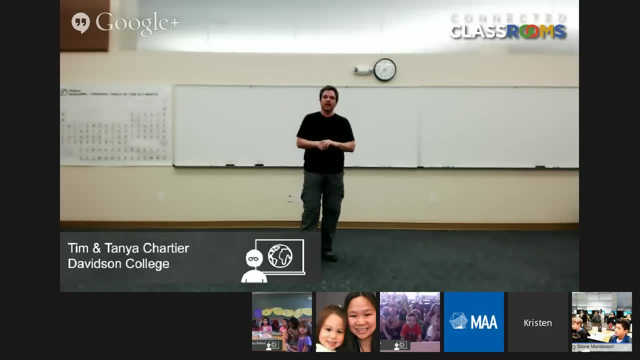 All right, Now we want to actually teach you an illusion, another illusion: the illusion of the ball. So I'll start: Take your hand out and grab a ball right like this: Put your hand in the seat and then throw it up and catch it. 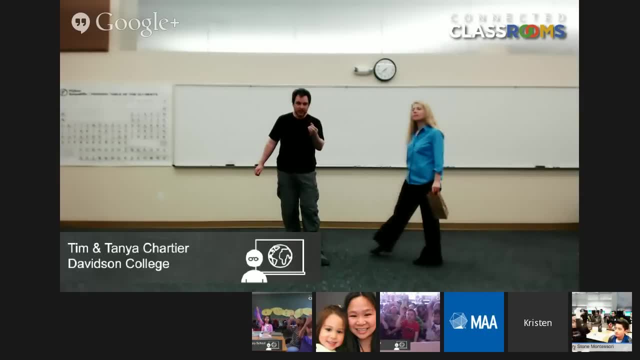 Good And throw it up and catch it, And now I'm going to toss it up and toss it to Tommy's hand, and then we'll see. So one of the important parts of the ball is that you watch it, and you watch it with your eyes. 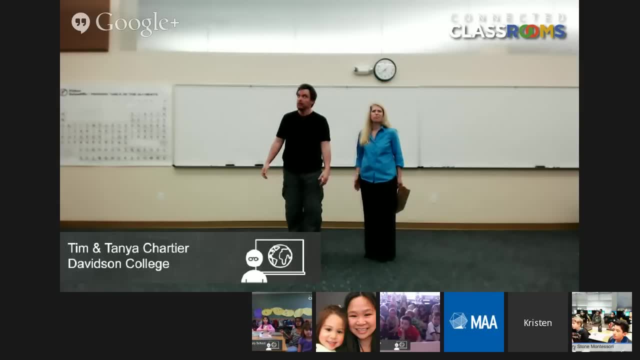 It's that that makes it look real. If you don't watch it, then where did it go? Well, maybe that was part of the joke, But that's what makes it look real is the more you watch and the more realistic the path or the motion. 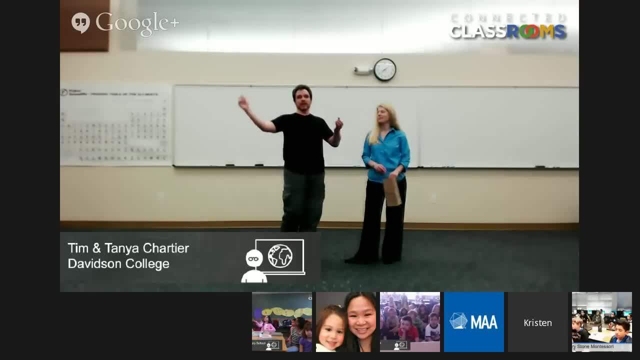 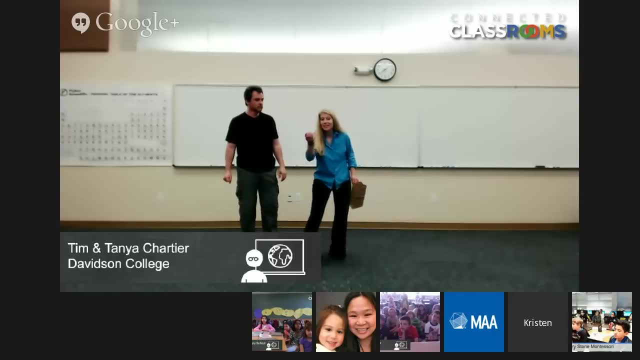 the more we talk about it in math, as you mathematically model it. So here you go, Tanya, Good, You can catch it and you can throw it, So you get a little weight. Watch it go up and watch it come down. 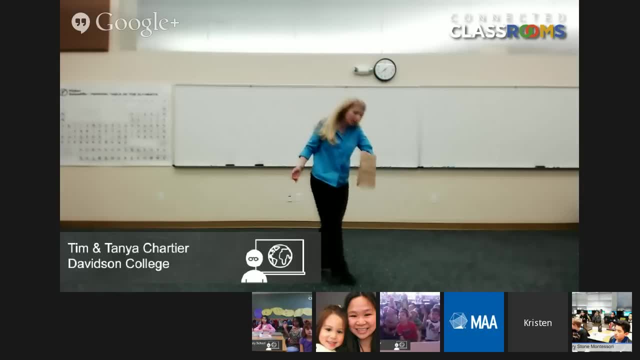 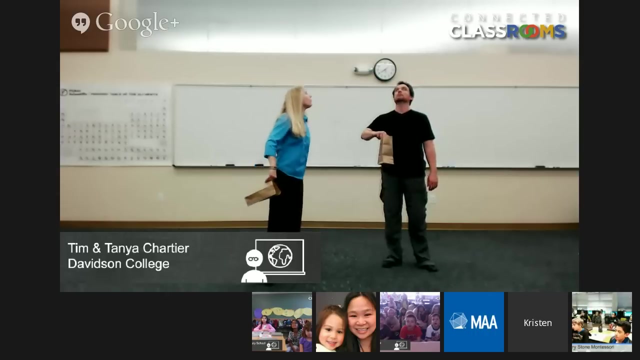 As you throw it up and you watch the trajectory, you can bring it back and it can land And that looks amazing. Whoa. Now how is that useful? I mean, other than it might look cool, how in the world is that used in everyday life? 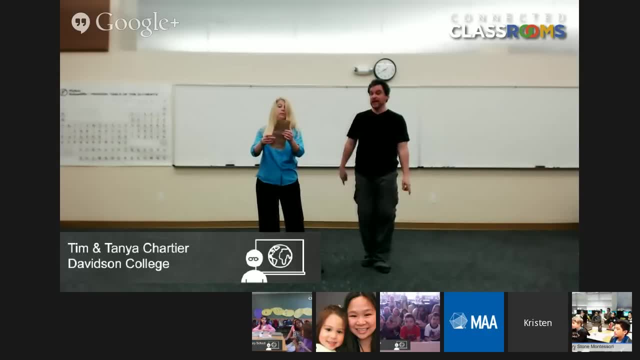 Well, it turns out that, first of all, some mathematicians actually engineered some great mathematicians. They actually studied how a soccer ball moved through the air and they actually discovered that the position that you put the ball in with the seams actually makes a difference in how it goes through the air. 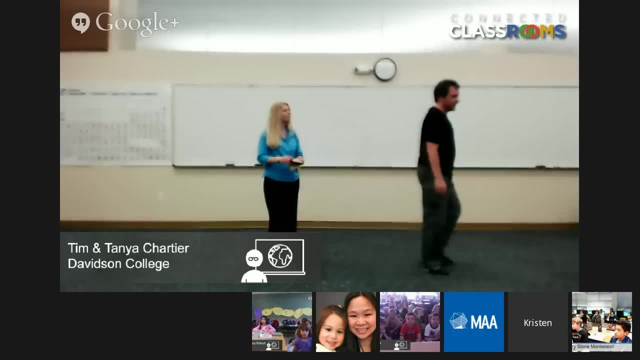 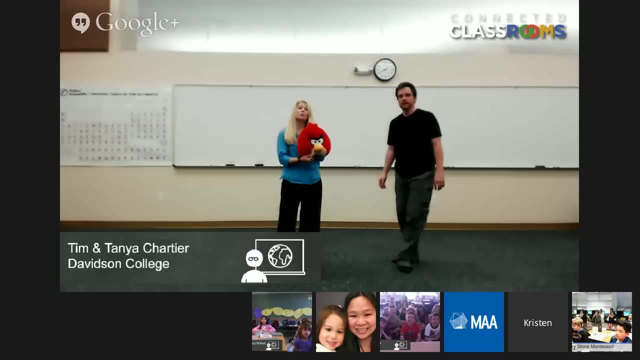 But there's another one. Another way that it's used is actually one that you've probably seen, and that's the way an angry bird is projected through the air. So every time you particularly use a red bird in those entry levels, it's math that determines. 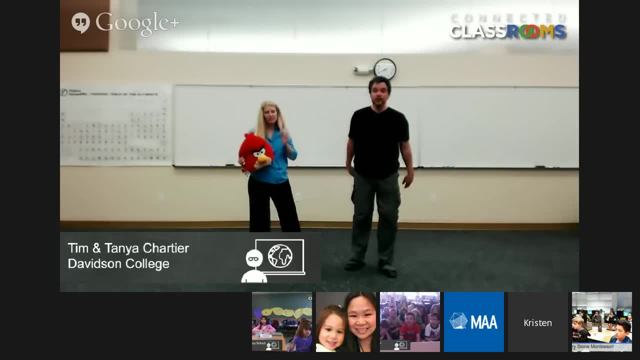 That curve And, depending on the classroom you're in, it's actually a parabola. If you don't know what that is, it's actually like that And it's actually math that helps determine that The other ones have it too. 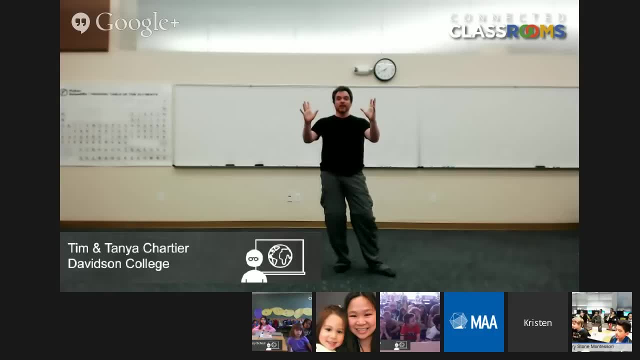 but some of them use more physics. All right, So now we've talked about math modeling, We've talked about the infinite. Now let's use some spatial thinking in a sketch. that is quite different. But see if you can see why we say: 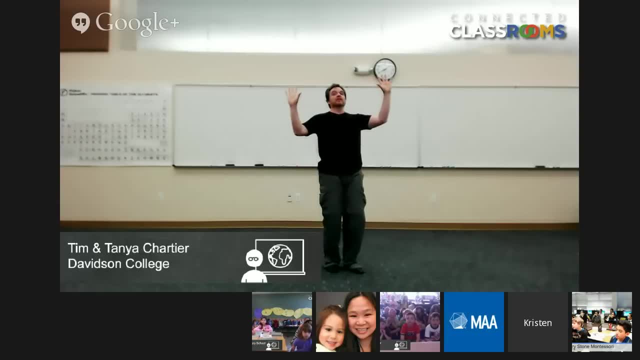 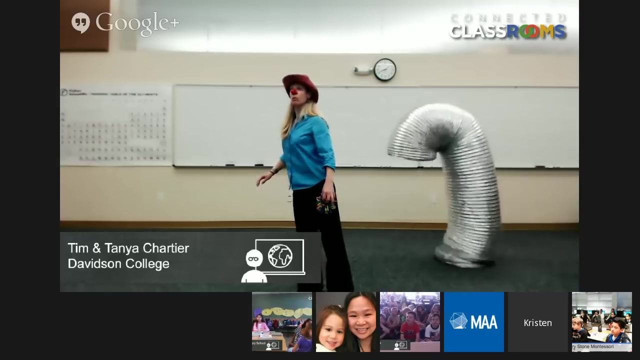 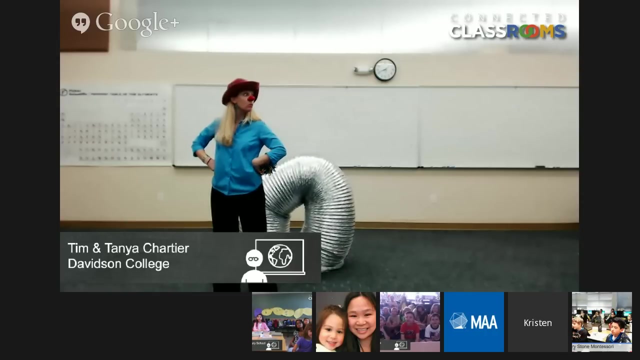 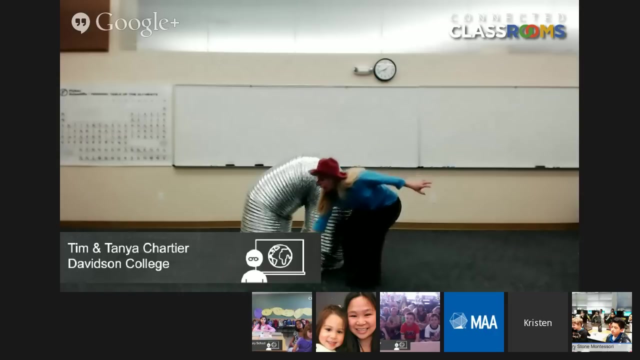 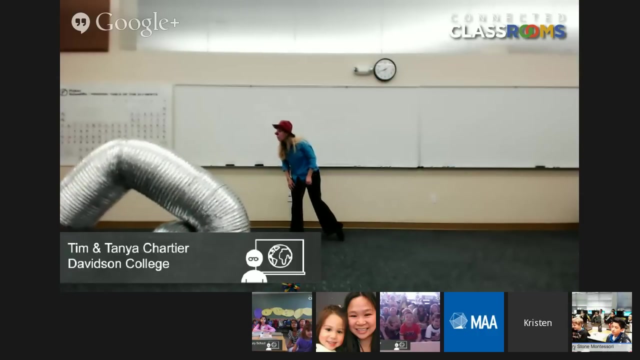 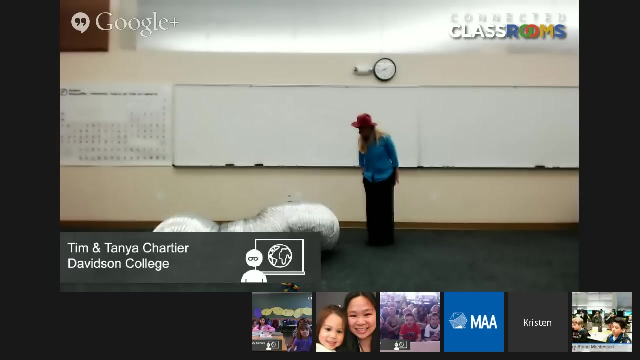 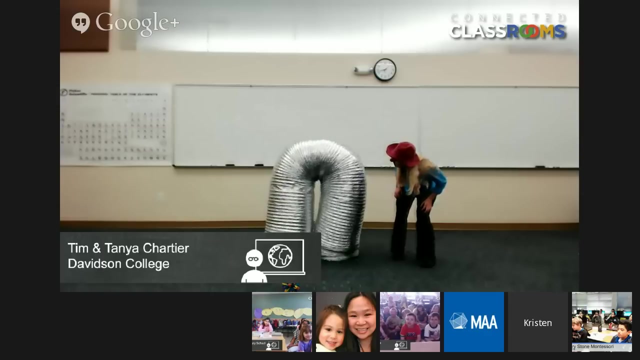 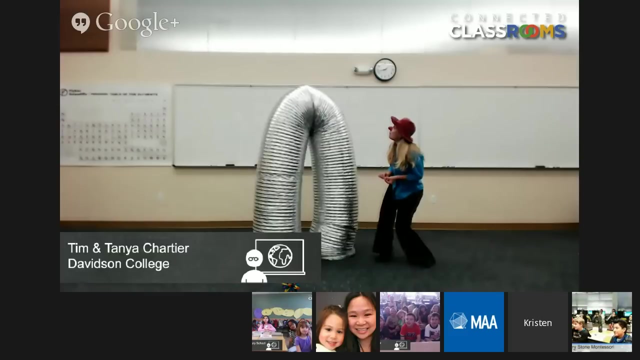 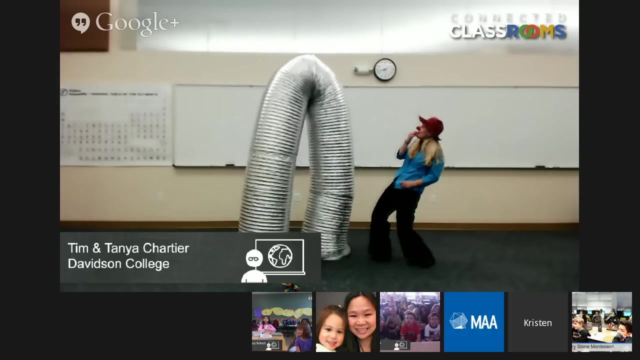 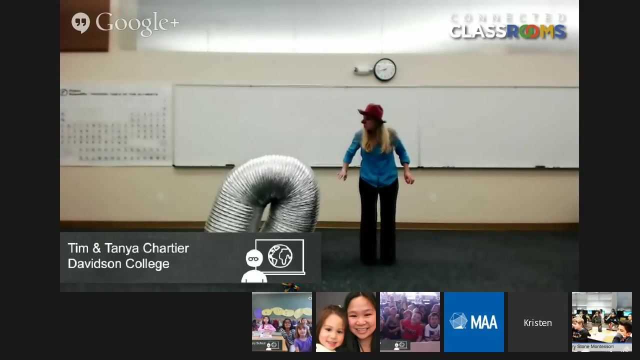 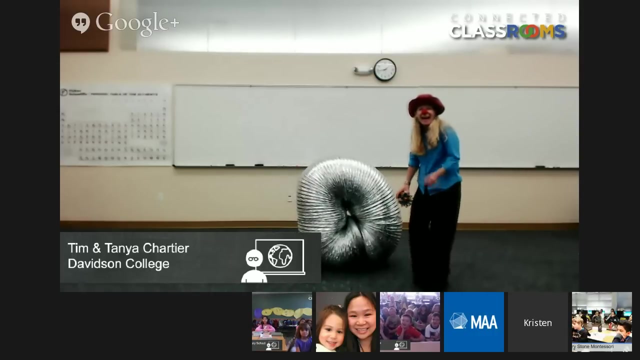 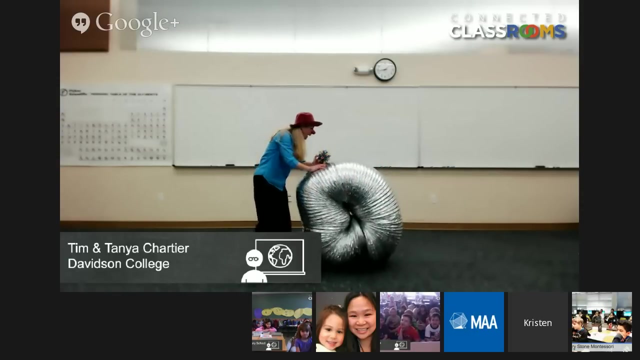 this uses mathematical thinking of space. If nothing else, it has a little bit of magic maybe in it, but it definitely has some mystery. All right, Here we go. This is some kind of observation, And that's the most important thing. 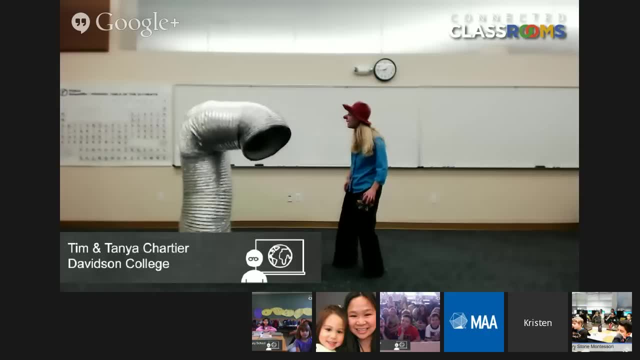 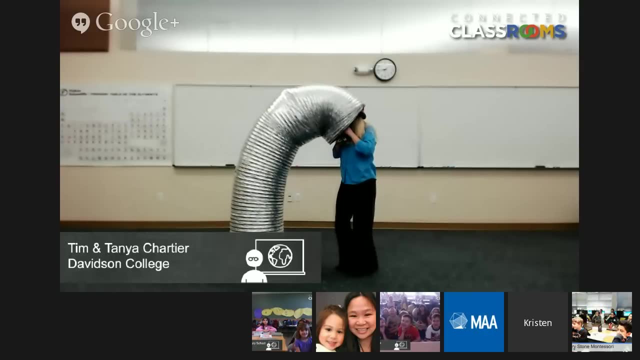 It's like I told you, For example, what's the first thing you do when you interact with a bird? Well, you're talking to it with the eyes. You're talking to it, So you look at it, You speak to it. 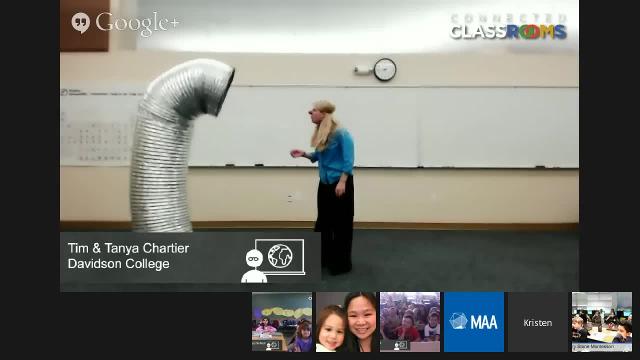 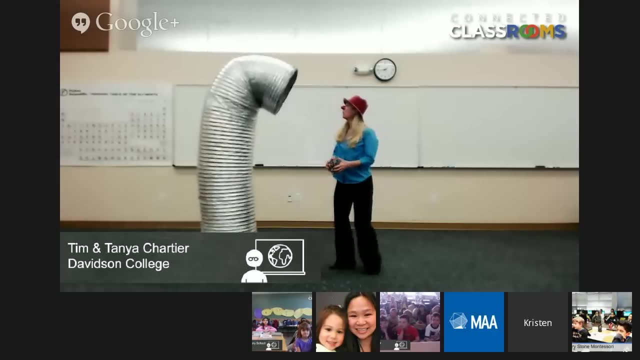 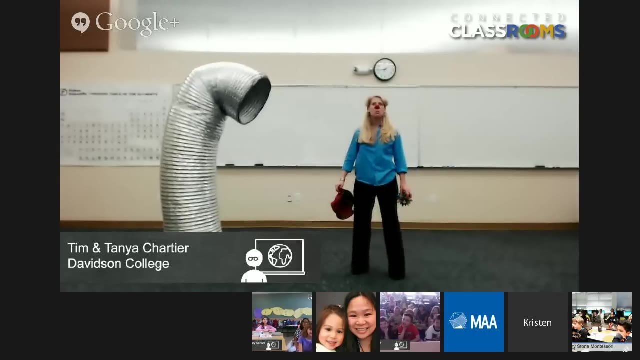 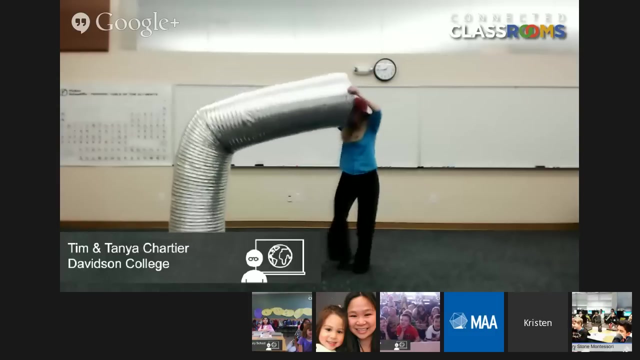 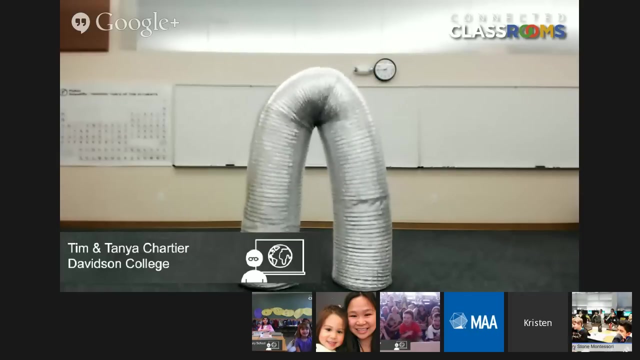 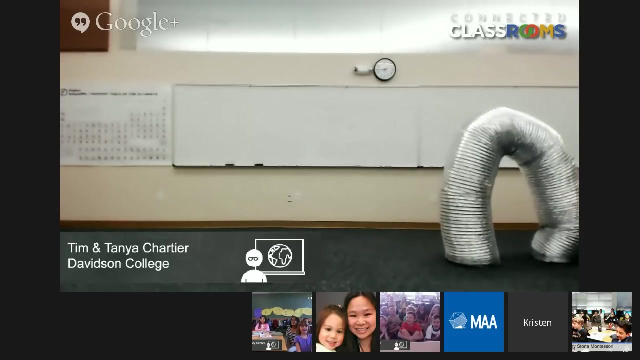 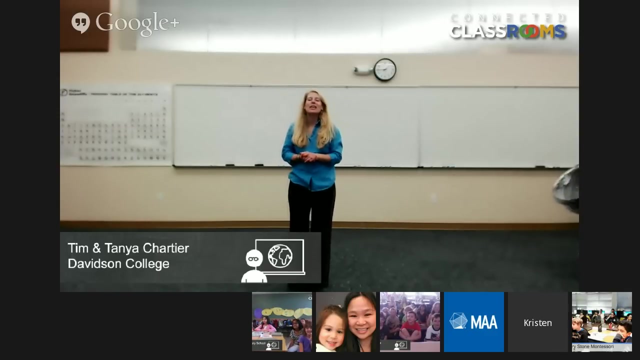 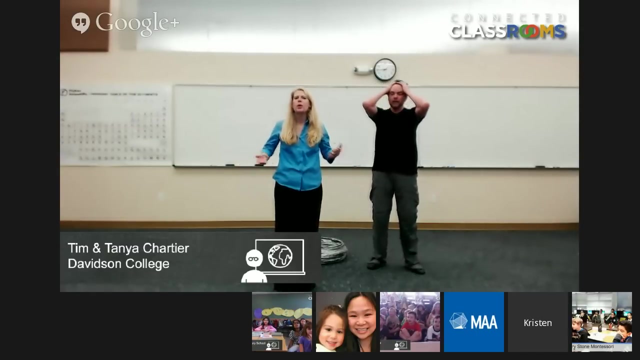 All right. All right, So that was a little bit different, wasn't it? So what we wanted you to take a moment to think about is where, in that slink- as we call him- or the tube, was Tim? We want to ask you to take a minute and use your spatial awareness and spatial thinking. 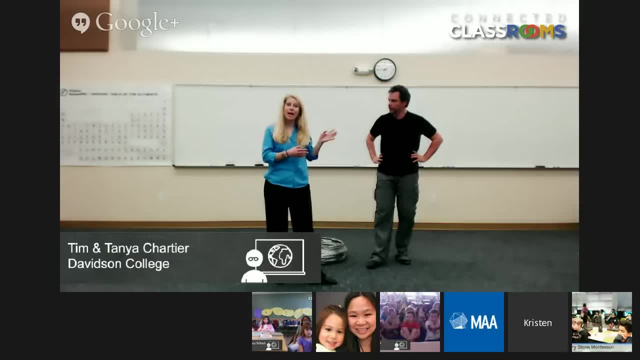 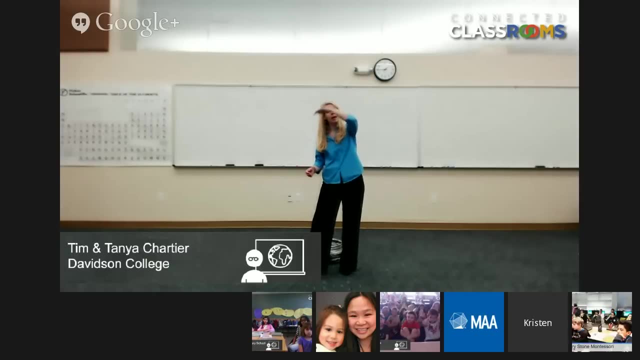 to think about. where was his body positioned inside of that tube? Let's think about a couple of these shapes. first of all, We think about the one that looks kind of like the parabola that Tim was talking about. We can see that his body. he's going to form it for us. 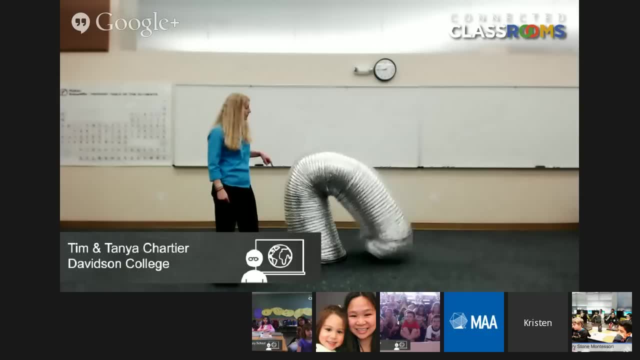 we can see how his body was inside of it. Here he is and what he is doing. I'm going to mimic the exact thing that he does, But first take a second. See where he is A beak here and his hands are down there. 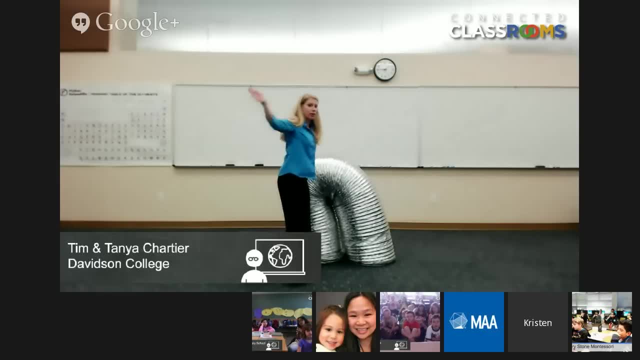 This one's a little easier, because you saw him get into it. You know that he's gone just like this, Pretty straightforward. But now let's let him move around for a moment. I'll kind of block him a little bit, Can you imagine? 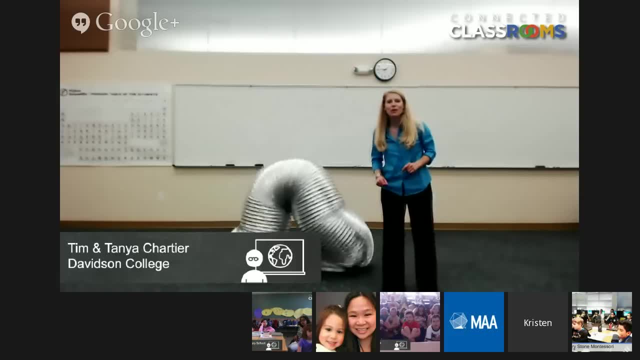 Keep track of it. Can you see Where is he? Can you move around a few times? Where's his head? Where's his feet? Where is his body? Okay, Are you a little confused now? What's up, What's down? 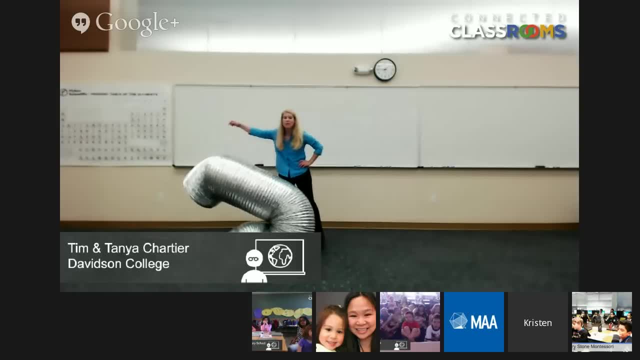 Well, we're going to reveal it for you. Make your guess first. What's here? Hands, Feet, Head. Think in your own mind or share in your classroom. Now I'm going to do the reveal. What do you see? 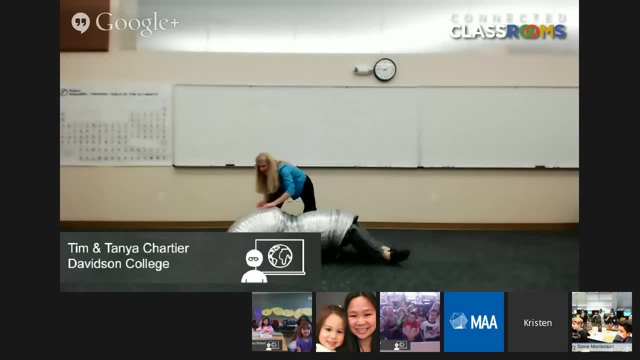 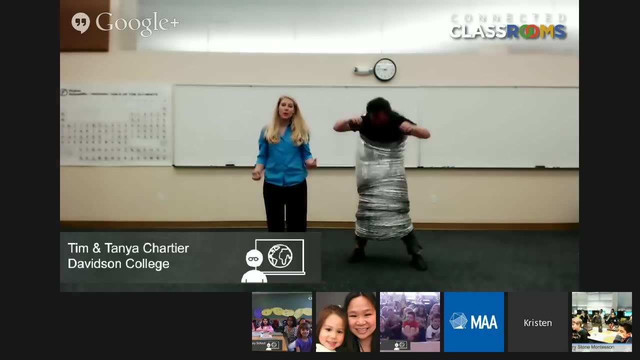 His feet. What do you see down here? His head. So there he is in that position. It's a fun one. And then the final one that we're going to give you a chance to look at is what happens when he's in that circular position. 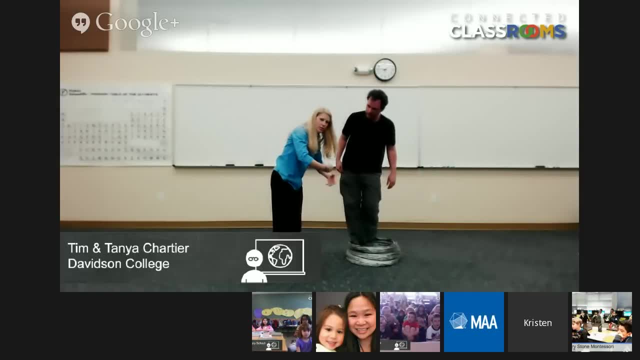 Now that one may not be too hard. but when he starts out, you see that he's in a circle And then he rolls. Well, Tim, I can guarantee, cannot do a somersault. So how did he do that? Well, that's the question. 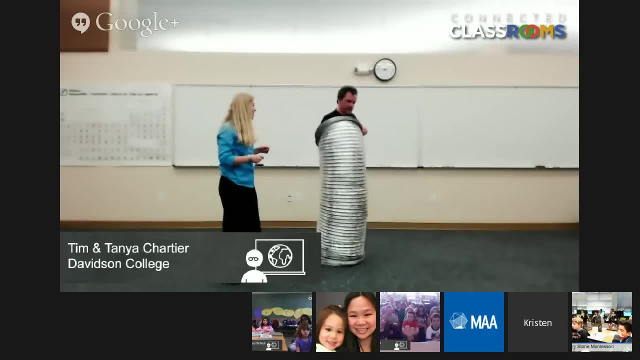 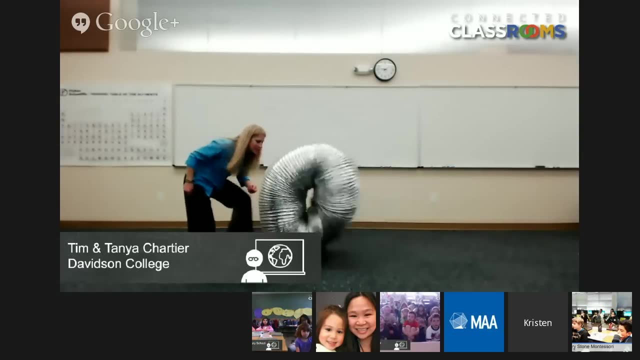 That's what you get the chance to see right here. Here he goes, Notice he's straight, And then he rolls, Notice he steps back with one of his feet. As he steps back with the other foot, he pushes some of the extra forward. 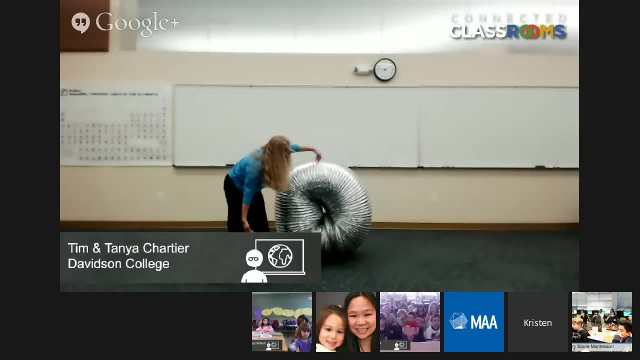 He puts his arm around and holds just his arm in this whole part of it, And it's his hands coming together that make it circular. So how does he roll? What does he do? Well, after my character gives him a little push, he just goes backwards and then comes. 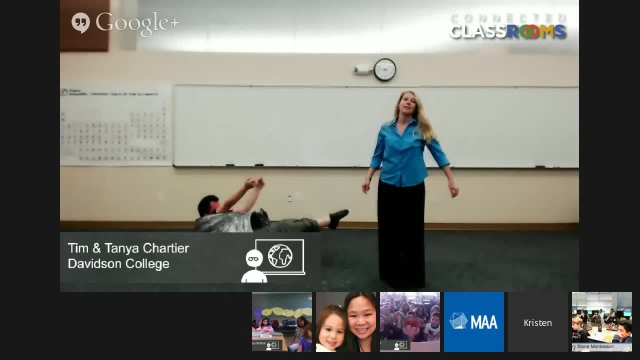 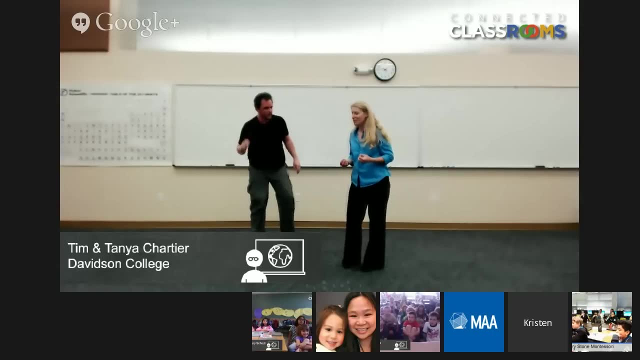 back up, come back up And it gets back up. that way, How did you do? How was your spatial awareness? It's kind of a fun game to play. I wanted to give you the opportunity to think about that and use that spatial awareness. 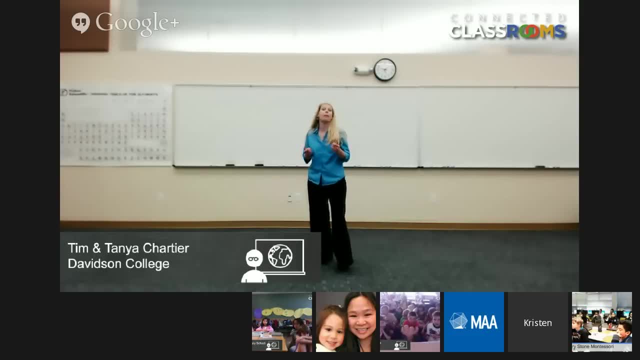 It's so beneficial. You think about what you're doing, perhaps in Minecraft and you're building. You have to think spatially or else you get disoriented. You have to think about which is what direction. Where did you build the last component of your house? 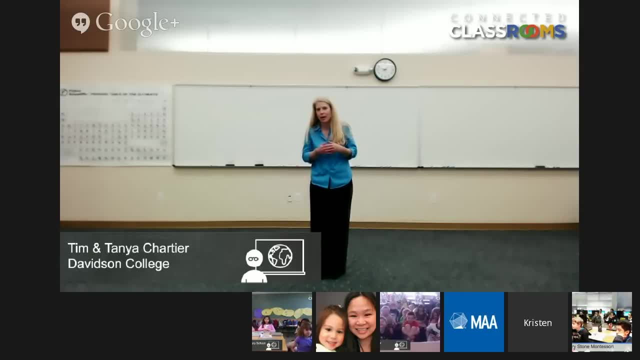 or perhaps where did you leave your animals that you were trying to care for or tend to? So those are all components that can help you think. spatial awareness Next. what we would like to do is I want you to think about mathematics a little bit differently. 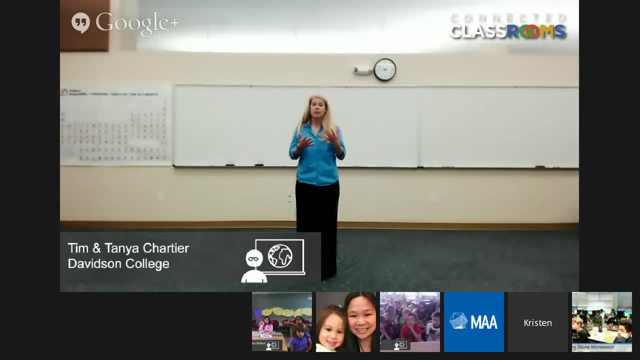 Some of you perhaps have already learned about the idea of division, the idea of taking a certain amount away and the idea of remainder. Well, I want to ask you: instead of thinking about remainder just as a number, I want you to think about the emotional side. 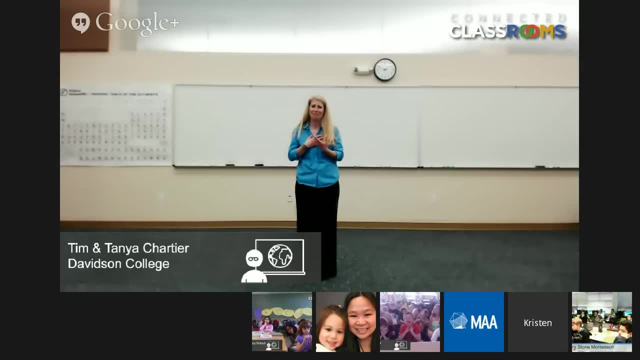 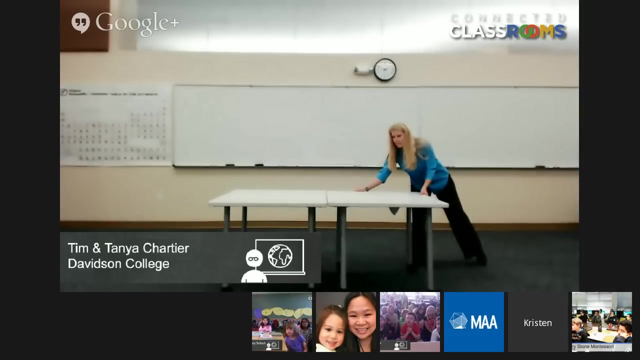 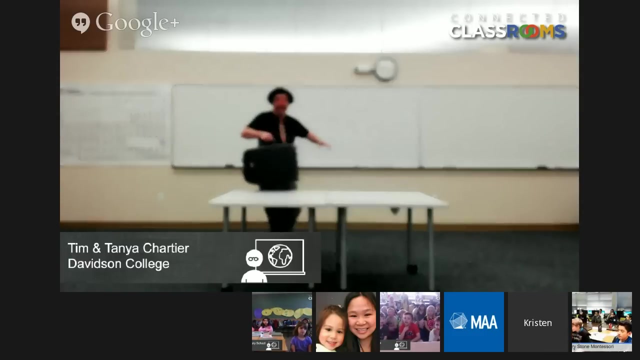 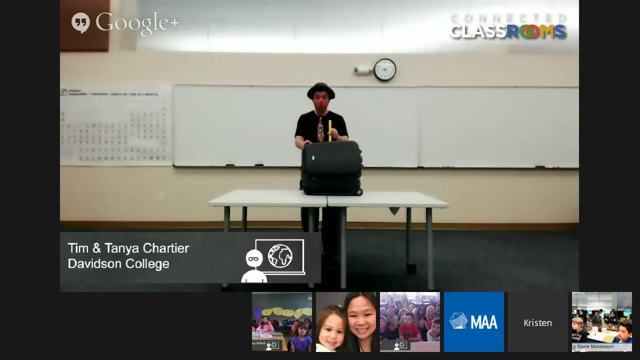 Of being a remainder and how that might feel to you. I'm going to leave you there and think about that as you watch this next sketch. Thank you, How about that? 3, 3, 4, 3, 4, 5, 1. 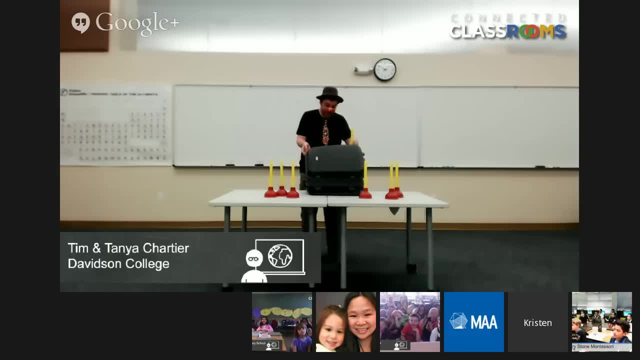 I don't know, I don't know, I don't know. So that's our sketch. on the remainder, Just for a little point, in your classroom you may want to watch this again. It's on YouTube. This whole Connected Classroom will be on YouTube. 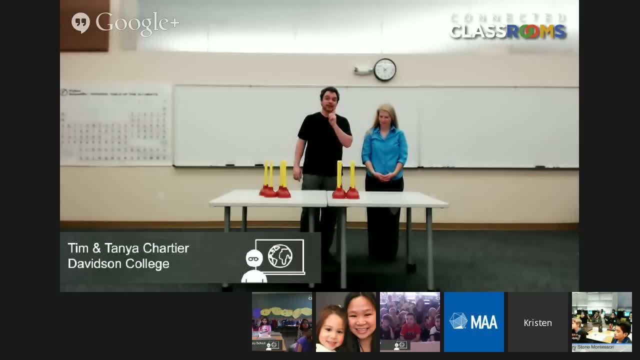 And if you watch this, it was specially designed so that I could not create a group without something extra. I mainly was working with odd and even numbers, but if you look carefully, I was actually also using prime numbers a lot, So it actually turned out. 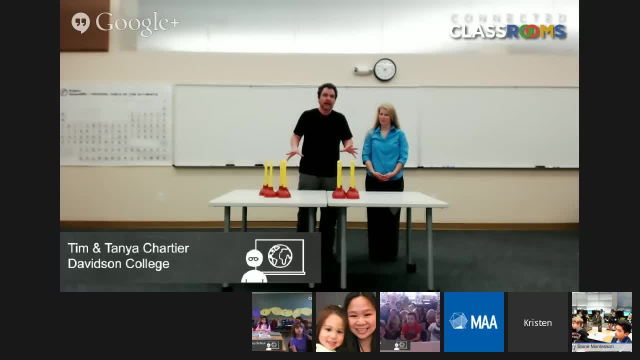 even if I decided to use three or four or five groups, I still would have something left over, And if you're not sure why, that's a good reason to look into it and look into why I said prime numbers. So let us move the tables away. 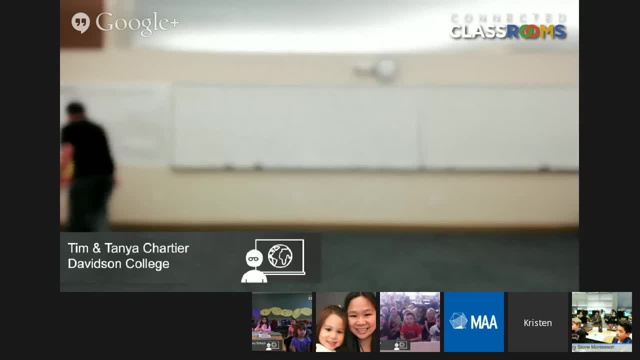 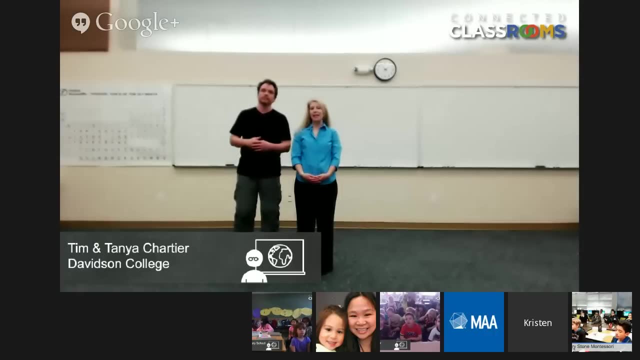 and we'll be right back. So let's move the tables away. So this is our way of integrating our interests into mathematics. We want you to think for a moment about how you can integrate your own ideas into the magic and mystery of mathematics. 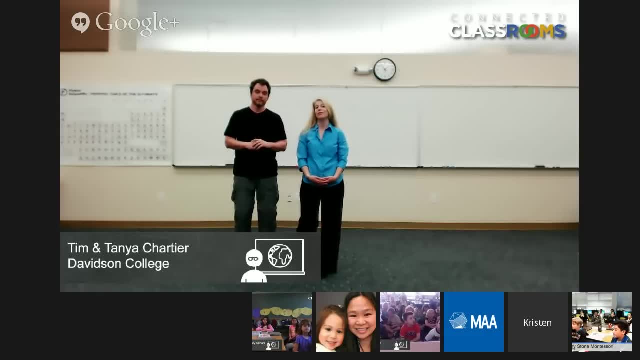 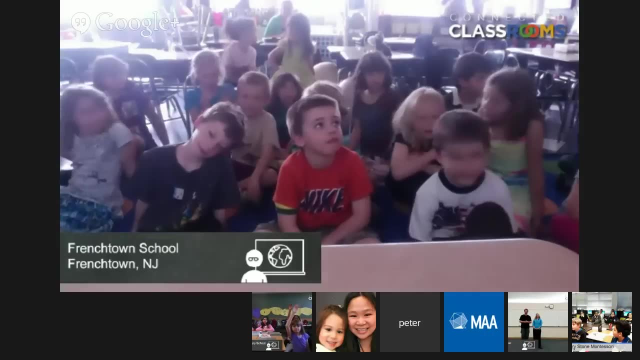 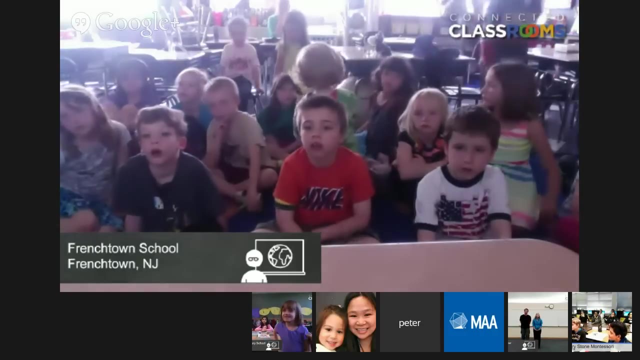 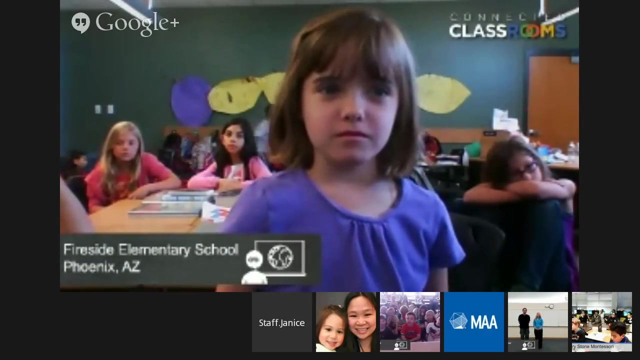 And so we want to open this up at this point to some questions from you. Don't be shy, We're here and we're ready, So we'll take them. So how do you relate math with other performing arts? Well, I don't do music. 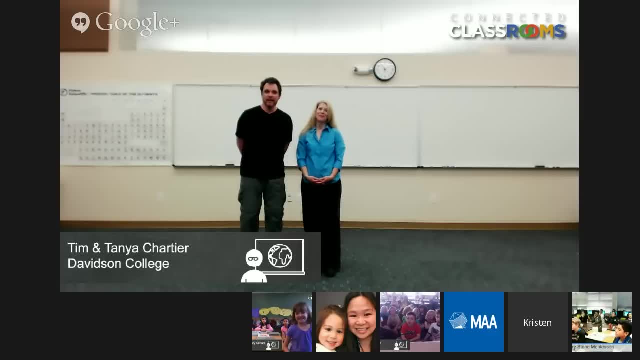 but everybody I know who does music talks an awful lot about using math in music. But I'm actually in a bell choir right now and I can guarantee you that being able to do math does not make you one of the best people in bell choir. 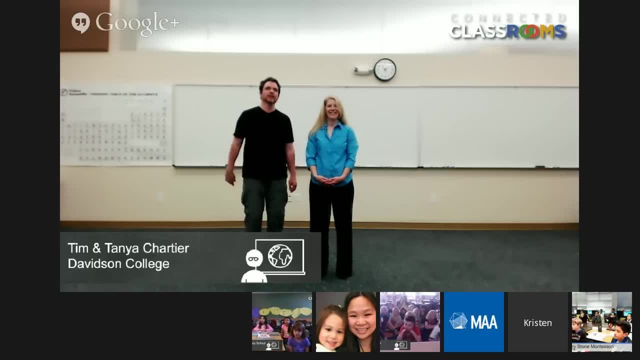 because I am definitely having a hard time, even though I'm very good at counting, But I know that it's used there a lot. Another place is actually juggling. There's something called sight-swap notation S-I-T-E, And it actually helped jugglers learn new patterns. 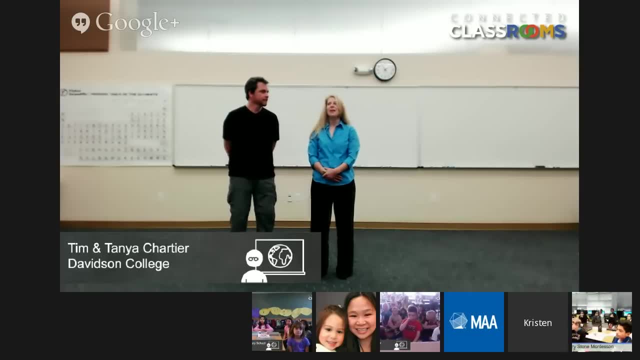 of juggling balls. That's a really cool one. Can you think of any For me? I think a lot of people think about music because of the commonality. I used to play the flute And so for me, I would often think about three-quarters notes. 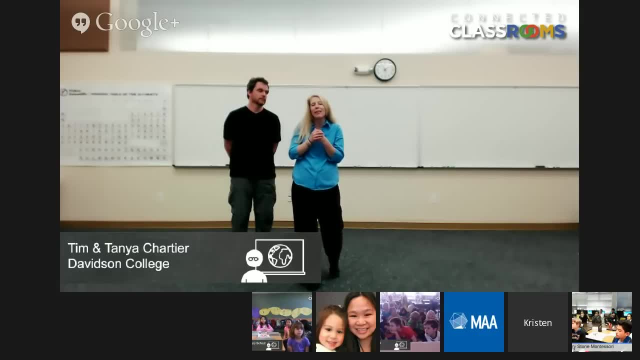 and thinking about the numerical components for that. That helped me a lot because when I played music it kind of helped me understand I'm holding kind of three-fourths of a whole note When I do a three-quarter note, So those kinds of things help me think about it mathematically. 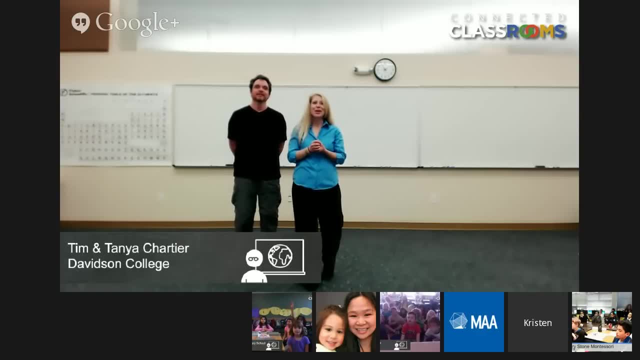 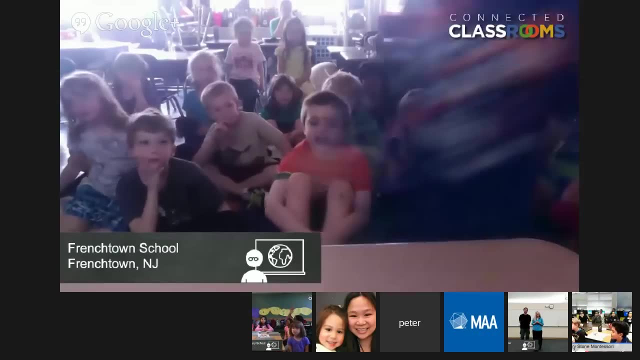 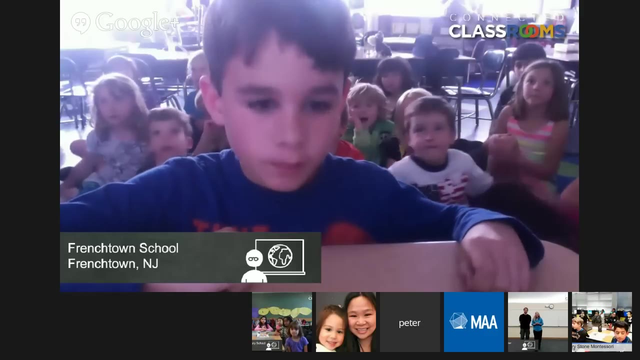 Hope that answers your question, sweetie. Does anyone else have a question? I see several hands. We need to turn the mute off of that one. I can hear you again. Who's ready? Howdy-do, Howdy-do, Howdy-do. 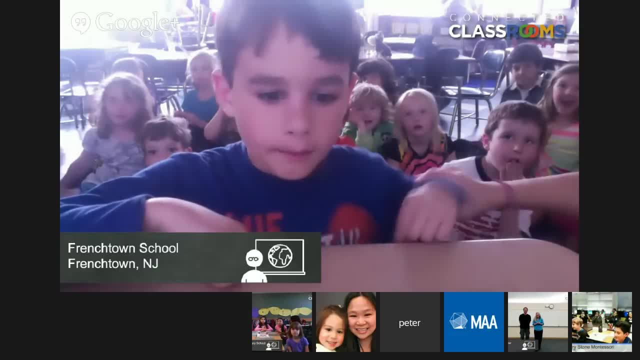 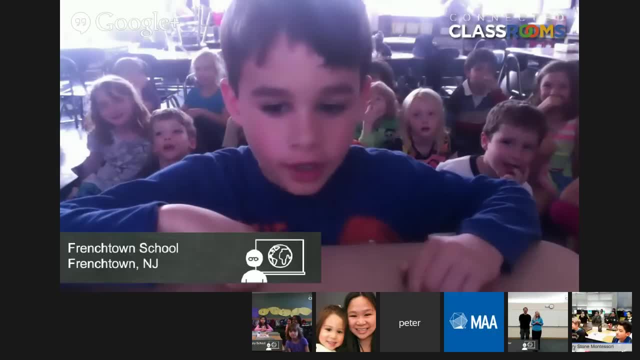 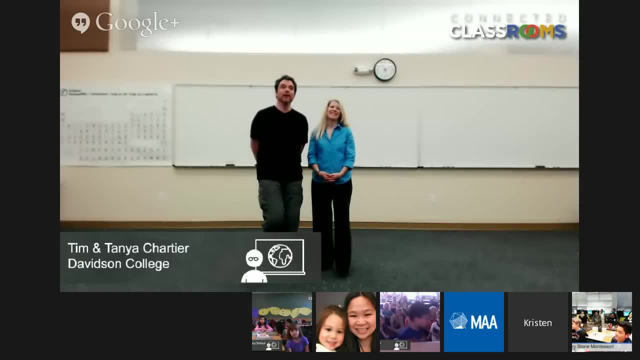 Howdy-do, Howdy-do, Howdy-do, Howdy-do. That's a great question. In math that's called a packing problem. There are a lot of people who, I'm sorry, thought we were moving to the side. 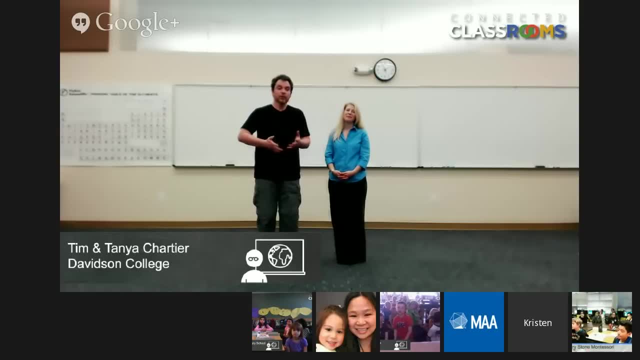 There were a lot of people who studied that for like. one of the questions is: if you were to take all the airplanes on an airplane carrier and put them on top, what would be the best way to lay those out Now? you asked about the plungers. 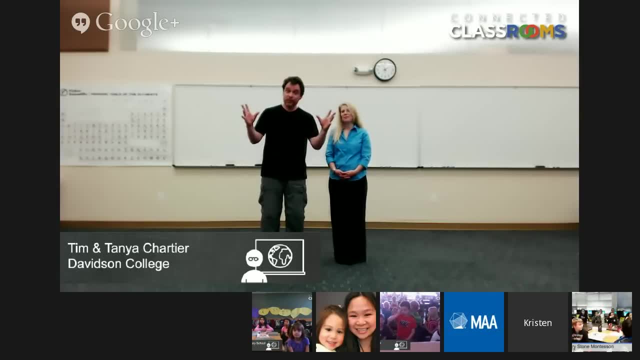 It turns out that what I did was I knew I had 13 plungers- There are 13 in all- and we just kept packing them until I found an arrangement that got them in. But you're right, They are very carefully packed. 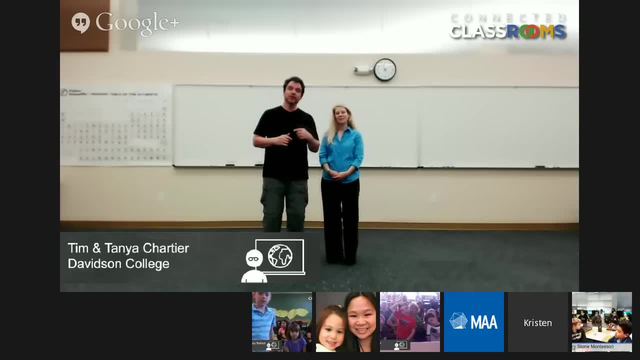 And in fact today, when we got them set up, Tanya turned to me and said: Tim, you need to pack the plungers because I'm the one who has that arrangement down. But basically there's research done by mathematicians, professional mathematicians, on packing. 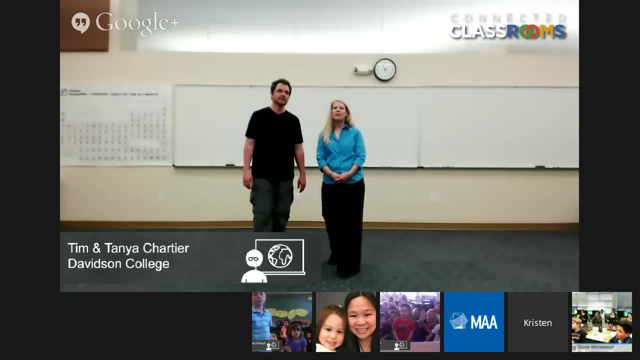 So it's kind of hard, which is probably what you picked up. There's also a really fun game out there. It's called Jump in the Trunk, I think is what it's called. It's about packing things into an actual little car. 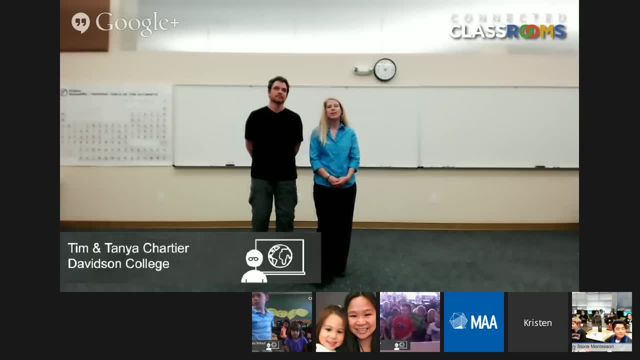 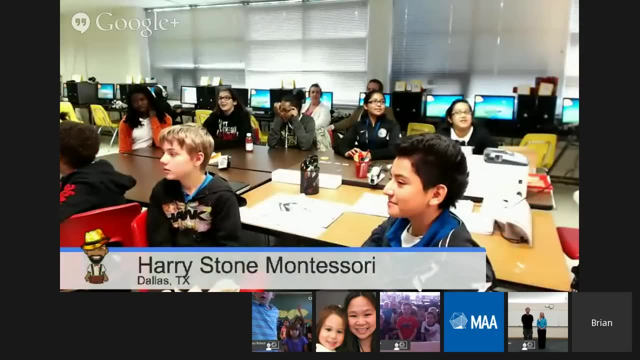 It's really adorable. We used to play it with our kids when they were younger, So you can go and check into that one. It's really fun. What's the next question? What is your favorite math concept to mine, To mine. 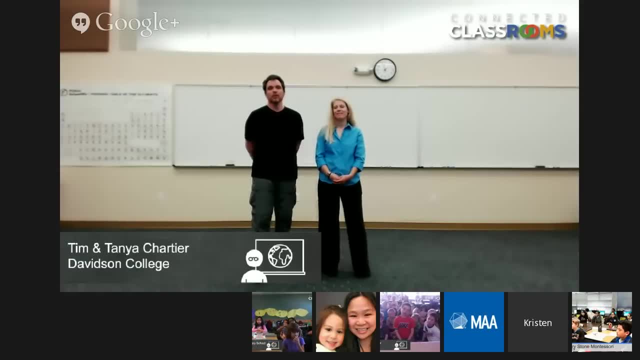 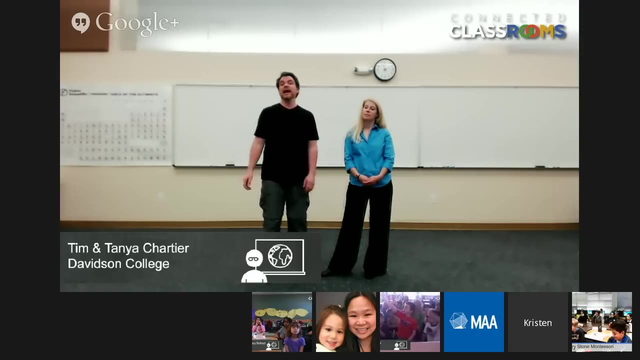 Huh, I think my favorite one probably is the infinite road, And I think it's my favorite because I can do it at any time without any props. So if somebody wants to see something, that's probably the easiest. Probably the one I think is the most mysterious is the bag that you saw. 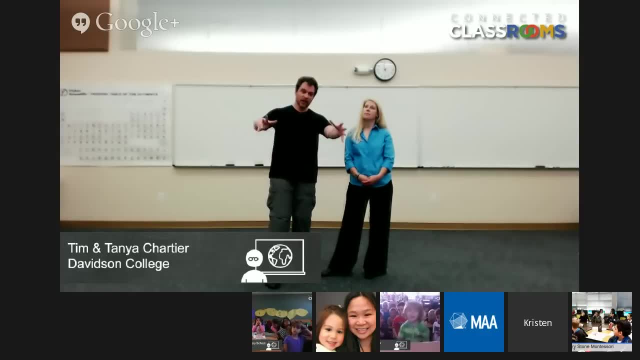 If we do it in street performing, there can be 100 to 150 people around us, all wanting to throw the ball. We couldn't really have you throw the ball, You kind of could, but it would be a little odd with your being in the virtual world. 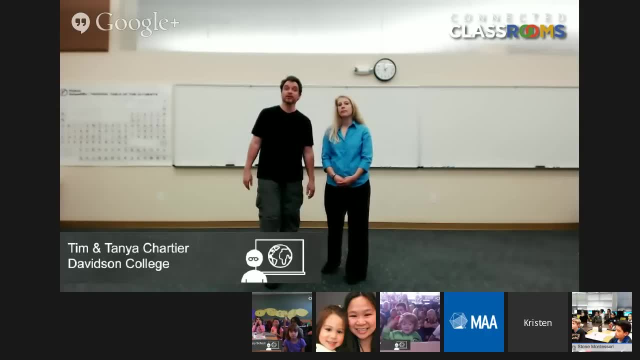 But if you were here we have. you throw the ball like I threw it to Tanya and that's a lot of fun. Usually kids your age will throw it really hard and Tanya's very funny. She'll always get stuck in the wall and things like that. 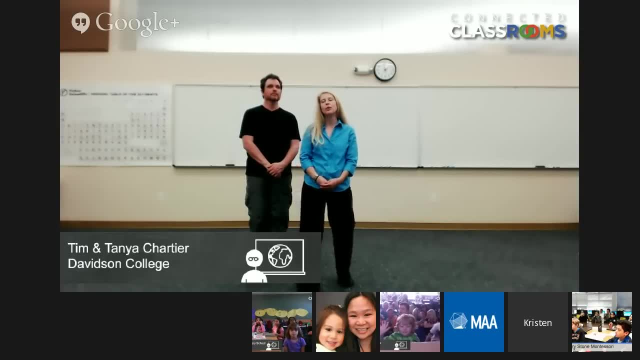 It's a lot of fun, I think. for me, one of the things I like to teach a lot- and you see, in performing- but unless you know what's happening in mine you don't realize it's there- is the idea of parallels. 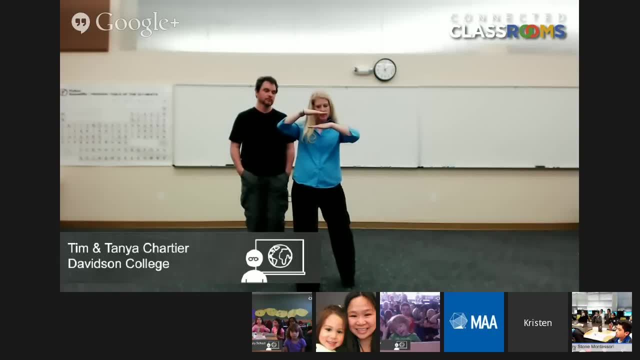 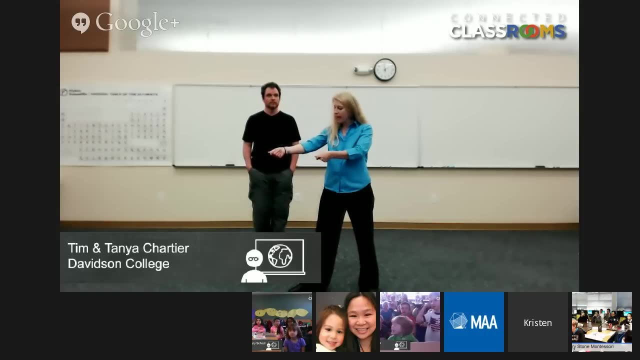 So you know that parallel lines are things that are kind of like this right, And when you teach the illusion of the road, we're doing parallels. If you could imagine a line, If you could imagine a line between this hand and this hand, there's a straight line right there and I'm pulling it this direction. 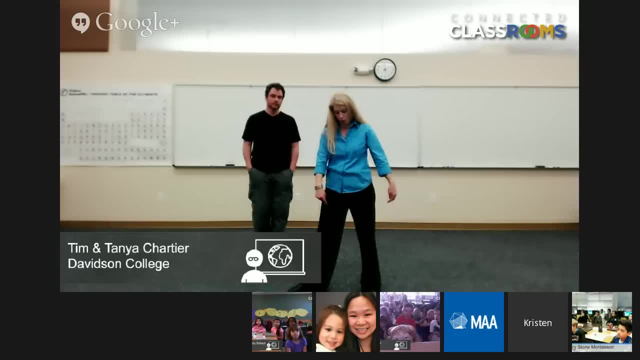 But if you look at my feet, there's a straight line between my feet or between my knees and they go the opposite direction. And in mine, all the time we're using opposite parallels, where there's movement on one part of our body going this way. 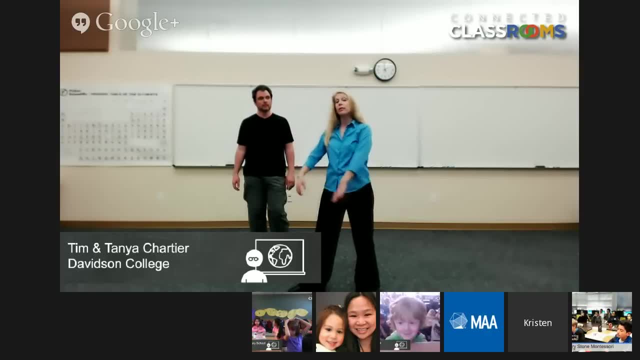 and on the other part of our body going this way, So they're opposite parallels. If you watch that, you can see my hands going one direction, my knees going the other direction. I love that Really quick. everybody just put your hands out in front of you. 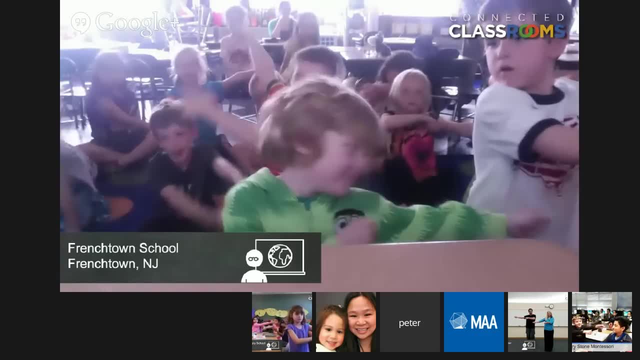 Just be careful. Be careful of the person near you. Now let's have Tanya teach you. There's something else in this called fixed point, So let's have Tanya. I'm not very good at teaching that part, so I'm going to have Tanya actually teach that to you. 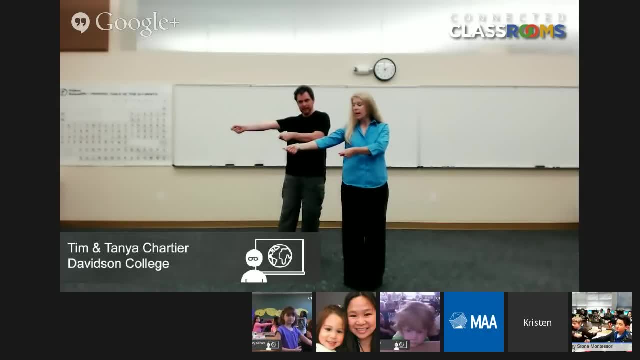 All right. So, Quentin, your hand is right here and this hand is right here, And the space between them is exactly stuck. All right, You cannot make that distance different, So you're going to try to pull it and keep that distance exactly the same in front of you. 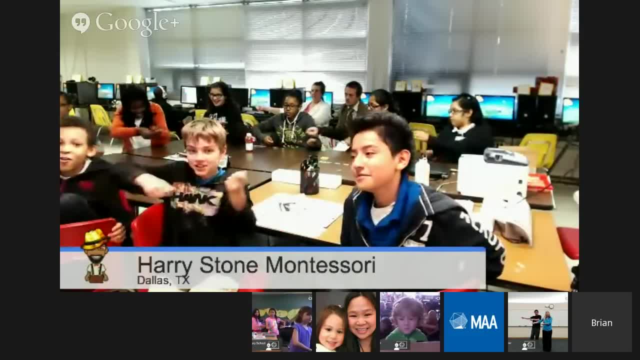 Good, Now we're going to go back out. Now I want you to see what happens if it's not the same. Watch. It's like I have a rubber band right here, Do you see it? I'm going to stretch it, stretch, stretch. 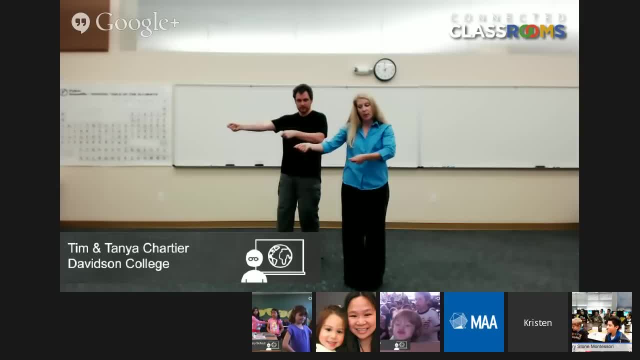 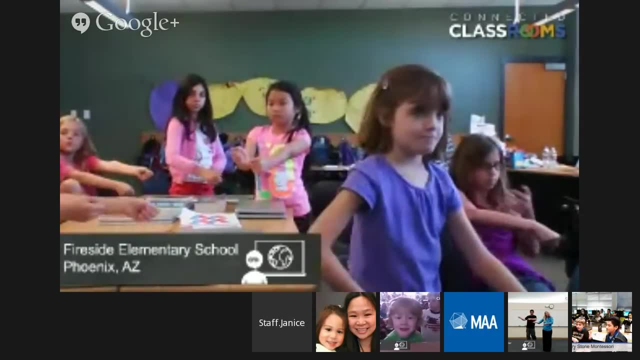 Now we're going to keep it the same and that's a taut rope, And now we're going to pull it and let go with your back hand and grab forward Good, Let go with your front hand and grab- Good, Pull it back. 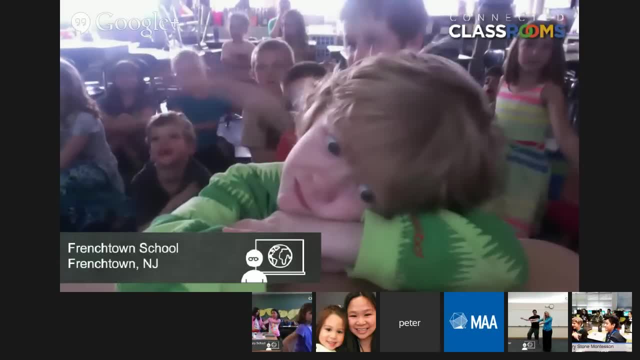 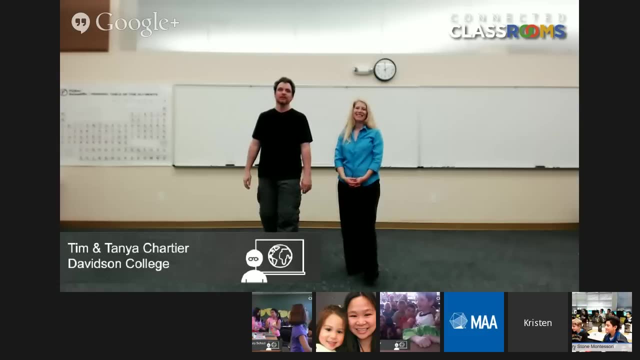 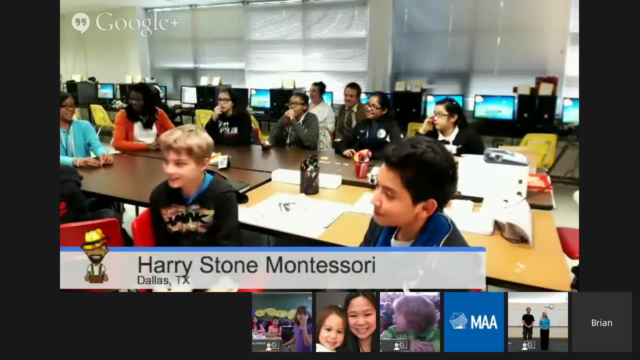 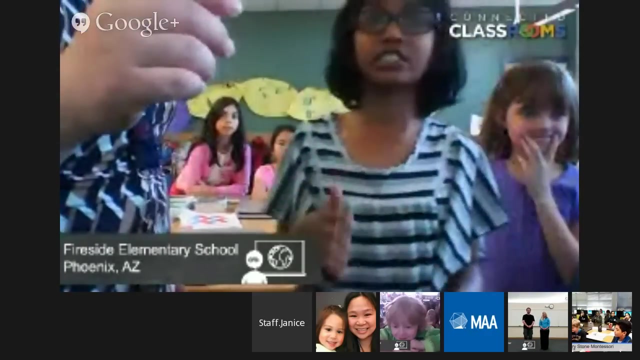 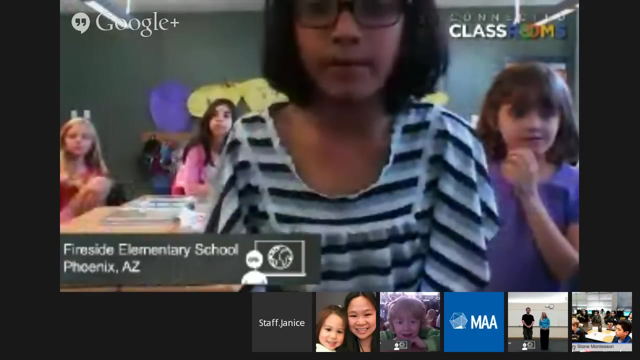 Let go with your back hand, Let go with your front hand, And they're both out there and you've got it. Then you pull Very nice, Grab, grab, pull. Very good, Good. Is there another question? How would you mine positive and negative numbers? 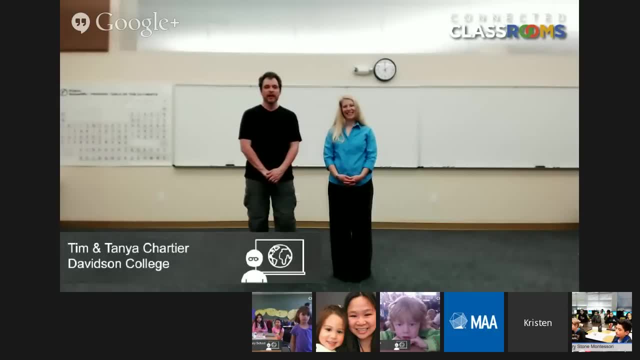 I was going to do positive and negative numbers at one time with a traffic light symbol that said walk, And so the positive would be positive and negative. The negative would be that you are trying to get across the street and then, when it goes negative, you have to go back. 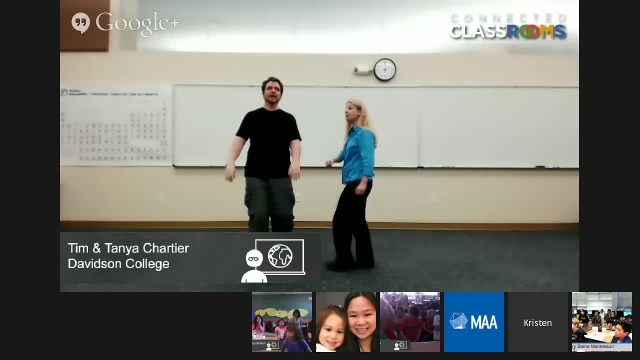 and then try to go forward and back, and forward and back. Another idea we had was actually using positive and negative numbers for going up and down stairs, But those ideas we've never actually taken to a performance level. No. So if you have ideas where that could make a fun sketch, I'm the only Tim in the math department at Davidson. 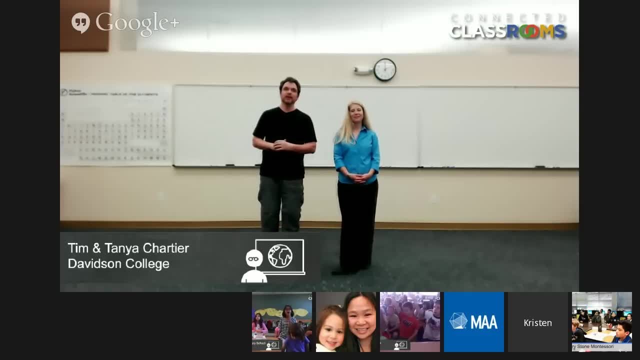 and so you could look me up, or you can look Tanya up, and you can e-mail us and tell us what your ideas are, because we're going to do a lot of work on that, Thank you, Thank you, We really would enjoy knowing. 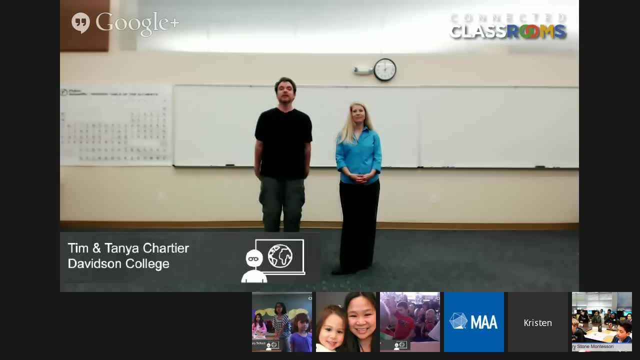 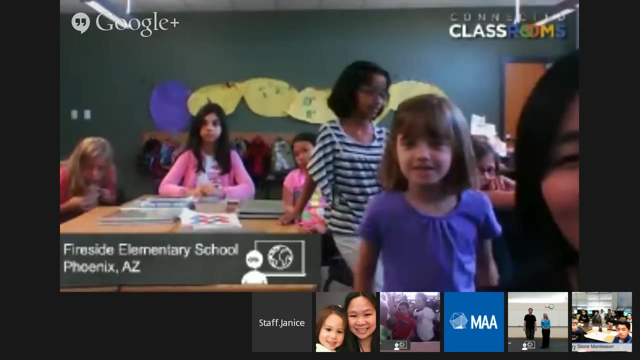 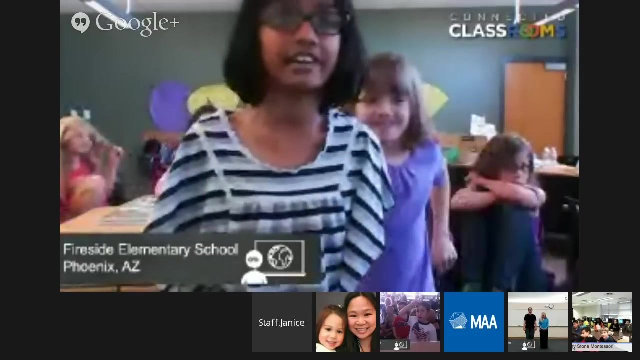 Sometimes it's someone coming up after a show or in a Google-connected classroom and telling us their ideas that help us figure out a way to perform it. But that's the ideas we have right now in positive and negative numbers. I already have an idea for positive and negative numbers. 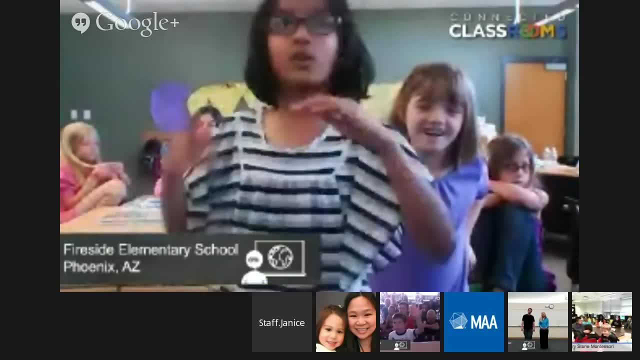 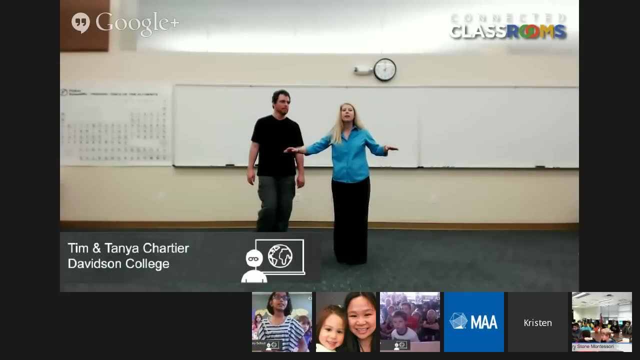 Okay, What's your idea? Elevators- Oh, that's a great one. If we had a nice curtain right here, we'd come and do that. That's such a fun illusion. You guys can do it. You have tables in your classroom. 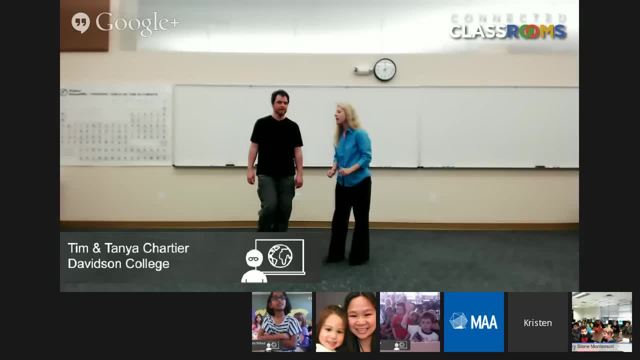 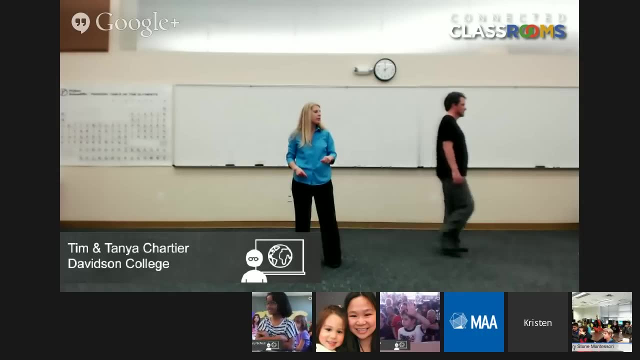 All you need to do is put like some coats or something hanging over the edge of them And maybe do a fake one. Can you pull one over real quick? A table Real quick. I'm going to have you block them out. 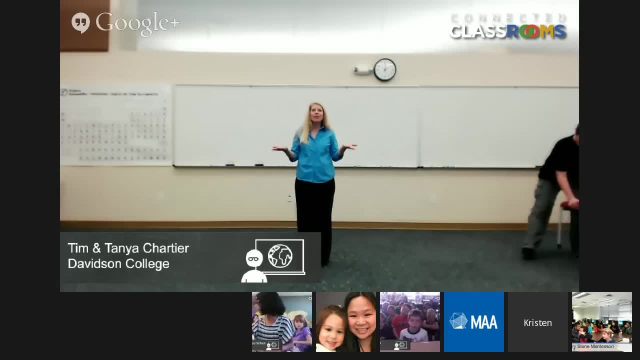 Or chair. That's fine. So Tim's going to grab one, And elevators are so, so simple in terms of an illusion. All you have to do is stand behind something Okay And you come up, Pretend like you're in an elevator. 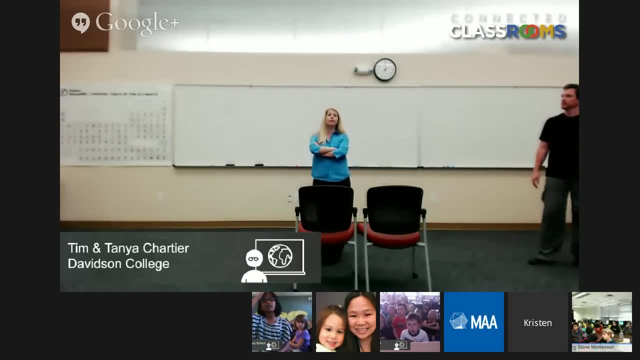 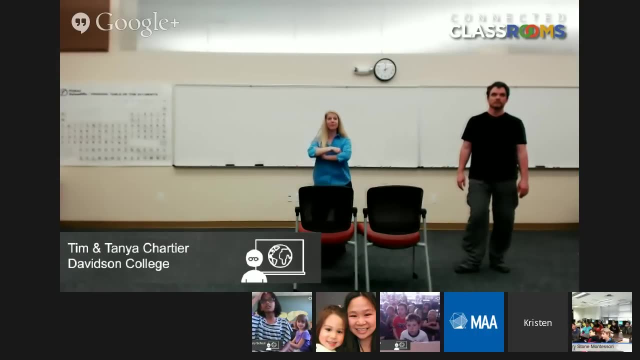 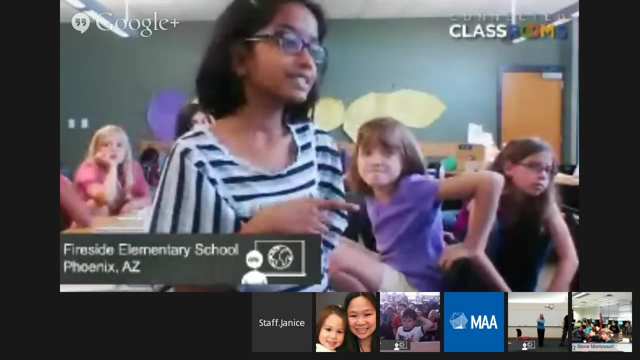 Push the button And then all you have to do is stand there And lower yourself down Right And then Awesome. Isn't that fun. Is that what you're thinking? That would be a great one Great idea. Just all I did was stand here. 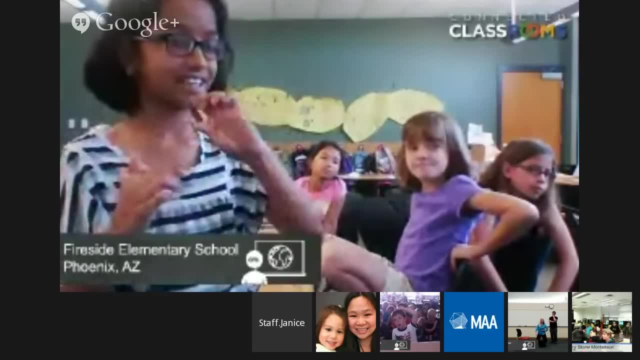 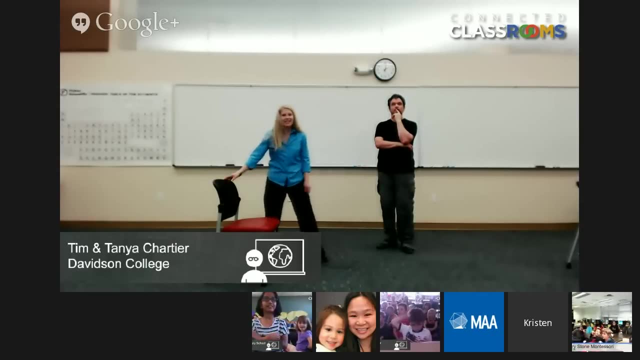 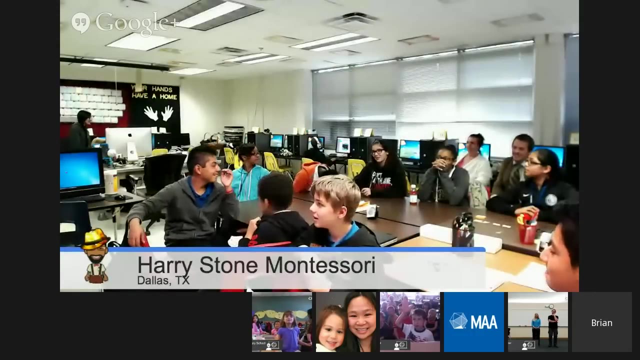 Keep this part of my body still, while this part of my body down here is going to change. Do you see that? And I keep this part the same. It's really fun, Excellent idea, Thank you. Thank you, That's going to be your stage. 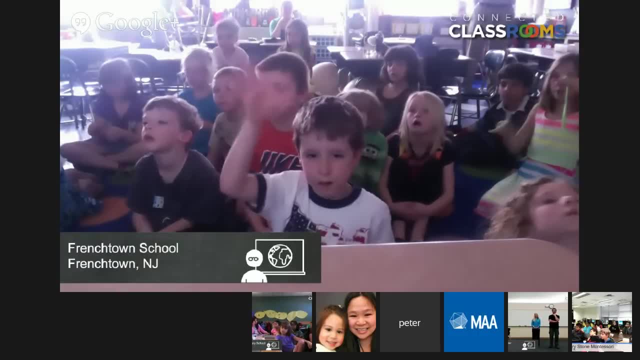 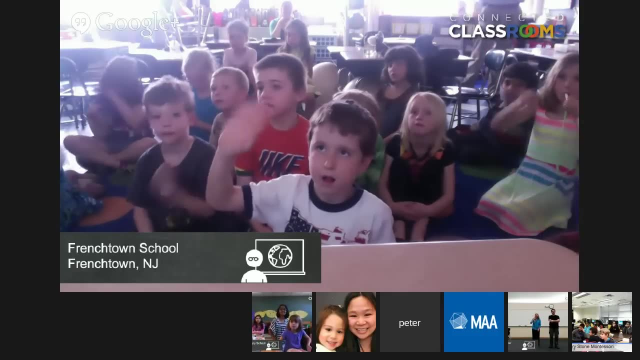 I can't do that illusion very well. It's fun doing it with stairs as well, But it would be a lot better when you have a curtain. I see another hand in another classroom Wave in: Hi, Hi, Go ahead, Go ahead. 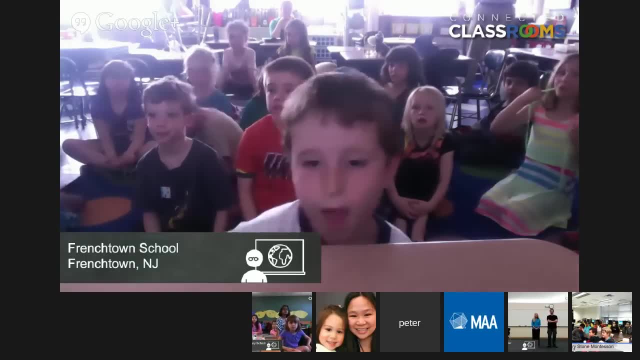 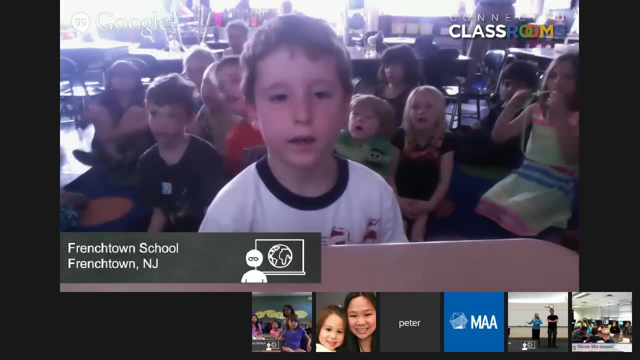 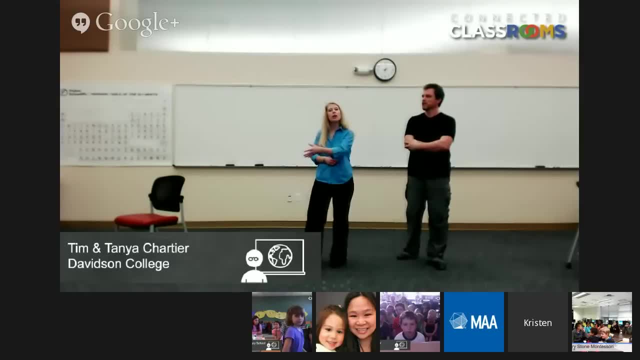 Okay. So when Tim was going, it looked like he was moving right when he was grabbing this, Is that what you mean? So he was pulling it and it's just like going really, really quickly. He kept going with the illusion. 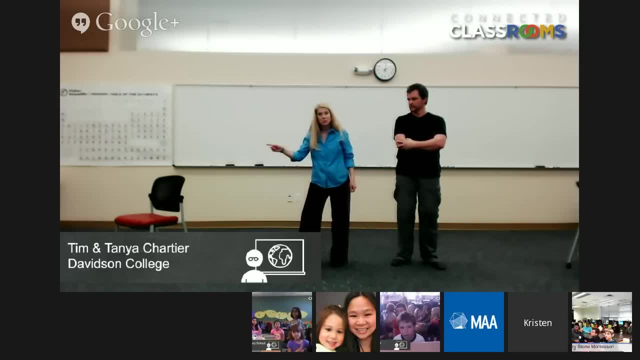 I'm only doing it with my hands. He started doing it with his legs. It looked like he was moving a little bit, didn't it? Let's have Tim step in here and do it. Is that the illusion? you mean, This one? 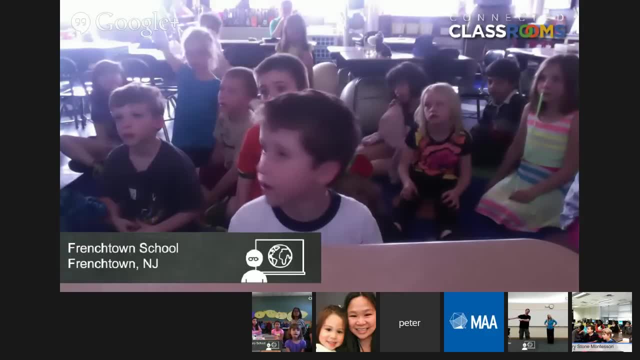 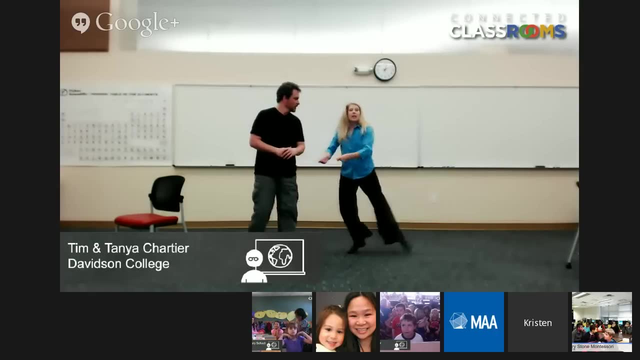 Is that the illusion you mean, sweetie? No, No, No, No, No. We get a lot of reverb in that classroom. That happens sometimes. We're going to assume that's what you mean. He keeps his feet going and he keeps. he goes really, really quickly. 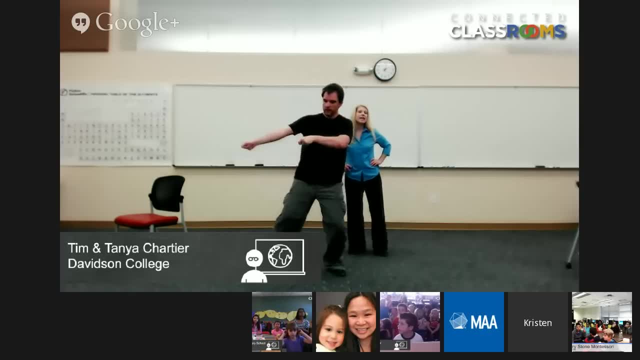 Oh, that's what I'm saying, Mm-hmm. Yeah, And it's just the idea of standing in place, Just like you learned to walk in place. I'm sure there have been times you just walked in place and exercised. 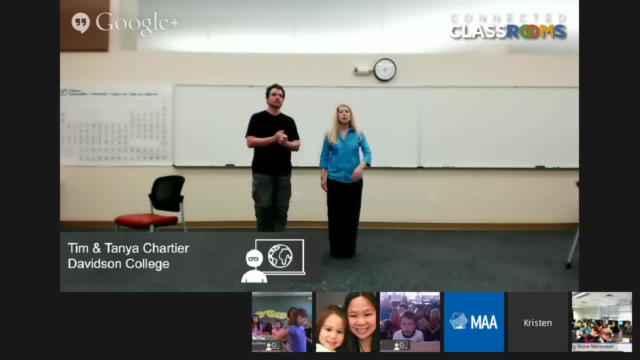 Well, an exercise exercising, Sometimes in gym. we used to have to do that, So perhaps that's what you were doing. He's just making it look like he's going somewhere. You can do the same thing with walking, where you're just taking steps in exactly the same place, but it looks. 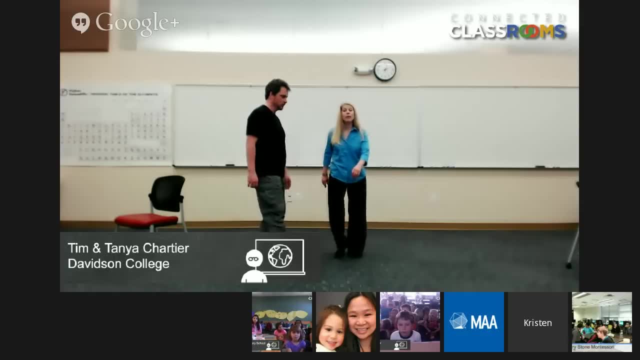 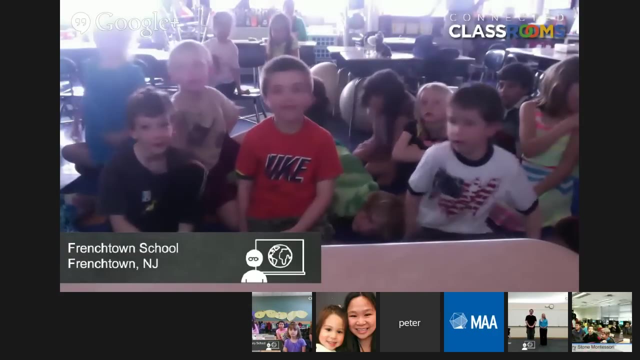 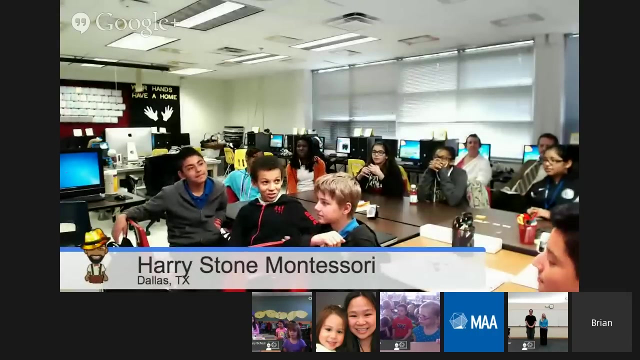 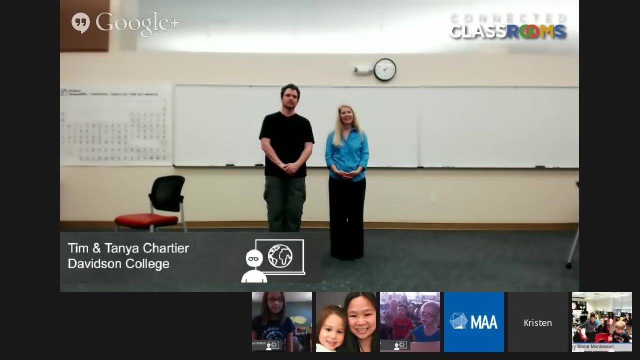 like you're moving somewhere, But our feet are just taking steps right where they are. We're not going anywhere at all. It's just the illusion of going somewhere. Okay, How would you mime percents? We didn't do that today, but this is the way I. 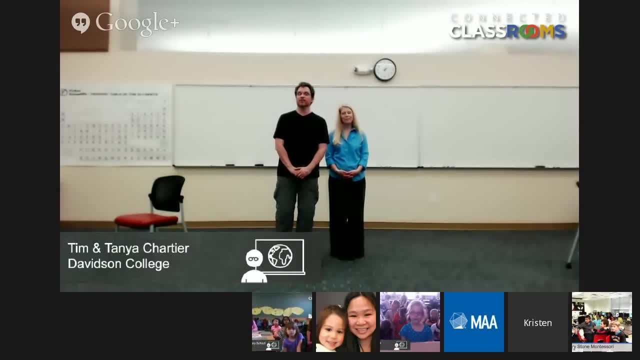 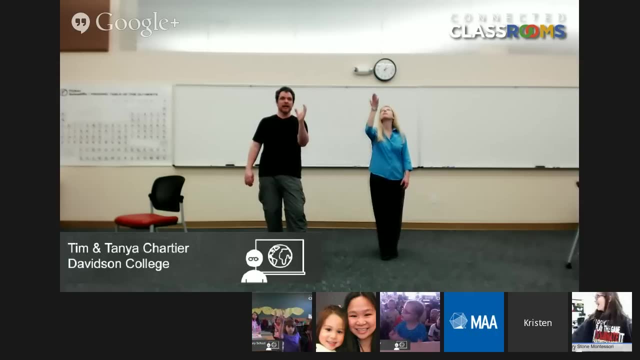 It's percent, but I usually think of it in terms of fractions, So I'll try to word it percent. So go out and grab a ball, like you did earlier. Just grab the one ball and throw it up and catch it Like that. Okay, Now it's mime, so go out and get another ball. 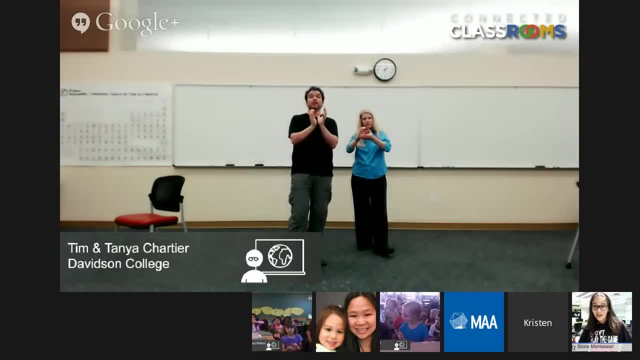 Okay, Put it together. It's mime, so you can mush it together. Now it's twice as heavy. So if you want to talk percent there, that's 200%, but if you're not at that point, don't worry about it, It's just twice as heavy. Now throw that up and catch it. 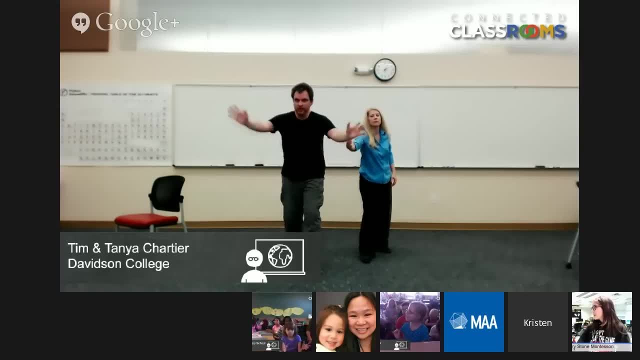 Good, Now put that aside and grab five balls from about the beginning. Make it into one. Now throw that up, Tana, and I won't do it yet You try it. Good, Throw it up and catch it. How heavy is it? 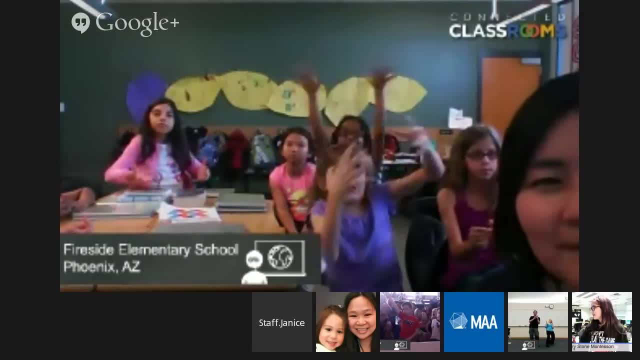 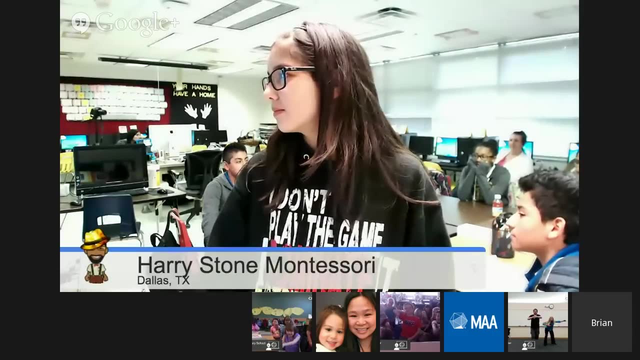 There you go, Throw it up and catch it. That was hard. There you go. I like mine. Then put it to the side, Then go out and get a hundred of the balls, Make it into one. Now it's too heavy, So push up. So now we're going to take. 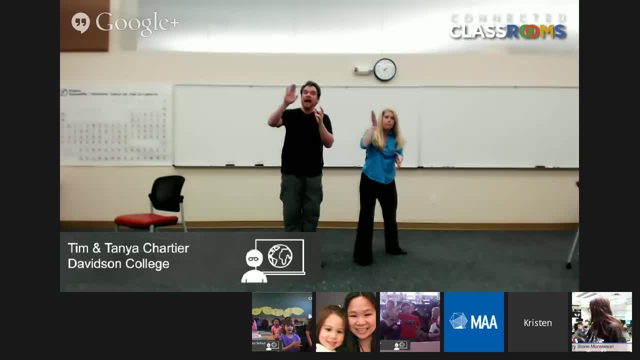 50% of it. So how much are we taking away? Half of it. There you go, Move it aside, Shape it into a ball. So now, how heavy is it? It's as heavy as 50 balls that we had at the beginning. 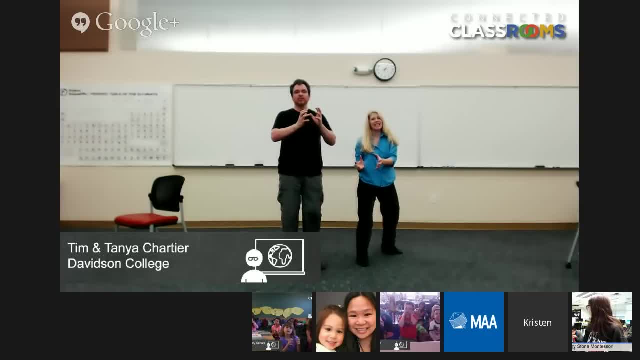 It's still too heavy, So try again. Trying means that you just make an ugly face and don't move your hands, So try again Now. take 50% of that away. That's half of it. Move it aside. How many balls is it as? 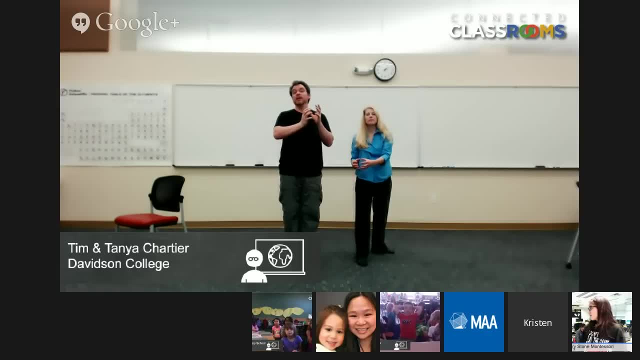 heavy as now 25.. Now we can keep going, but let's just stop here, because it keeps us on whole values. Pick that up Now on the count of three. you're going to throw the ball way up and throw it out and ever on. All right, It's mine, so we're just recycling, So ready. 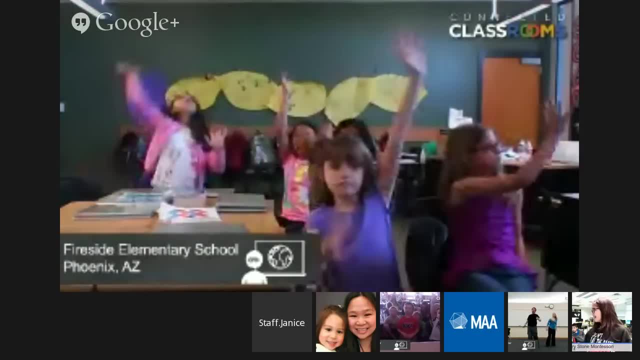 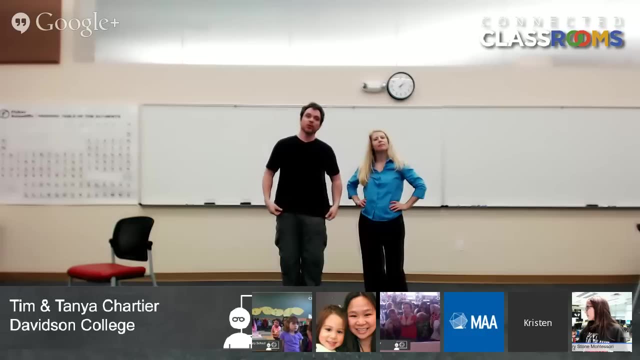 One, two, three, four, Like that. That's the way we do percents. You might come up with another way, but that's one that we like to do to show fractions of our percents, which I think of in the same. 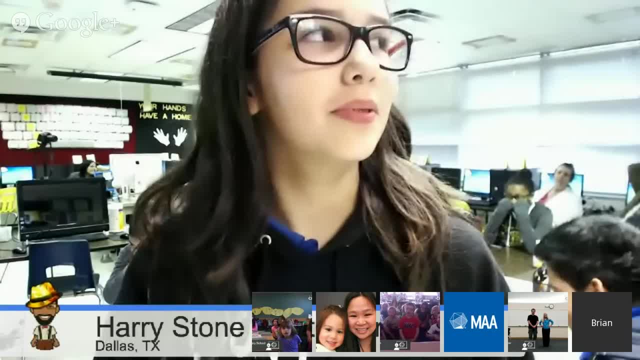 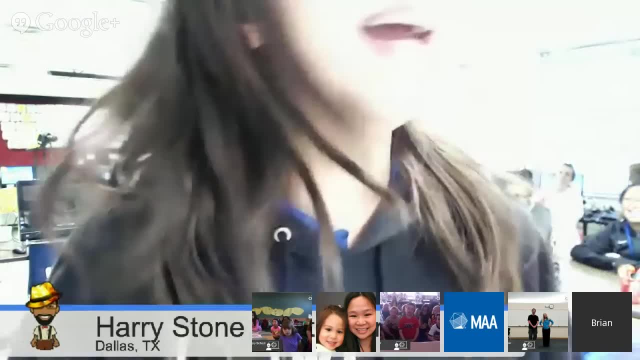 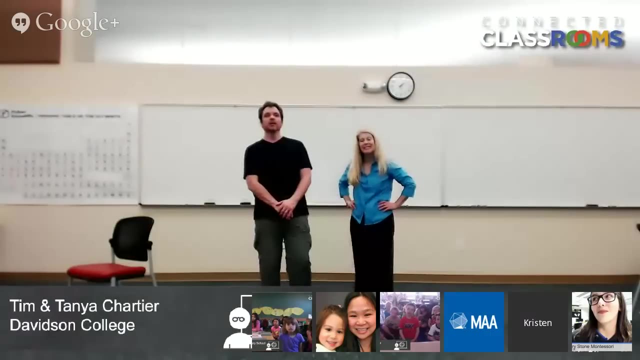 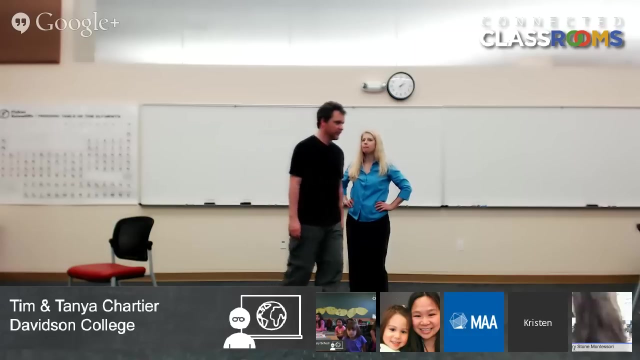 way. Do I ask it? What was your question? How do you interpretate science into it? You're on, Do I? Okay, How do you interpret science into this, into this? one idea is is when you use fixed-point like if you wanted the angry. 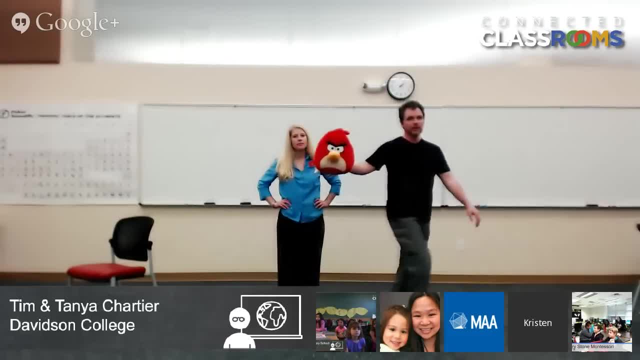 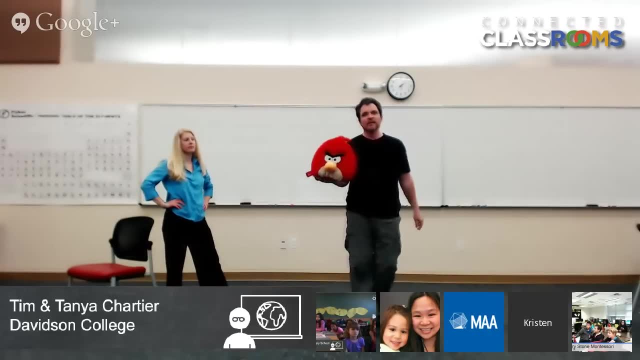 bird to get stuck. you can walk with the angry bird and have it get stuck, and then you push it, and then push it, and then push it like that. so there's a lot of physics in there that you're using. if you're not careful, you can make it. you. 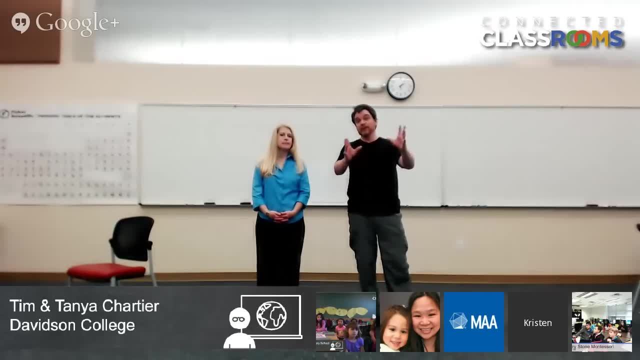 can make it non-physical, but if you go too far from what the physical world looks like, it doesn't look real. and so really a lot of physics in there. probably the only chemistry in there is the fact that we sweat. so that's about all I can. 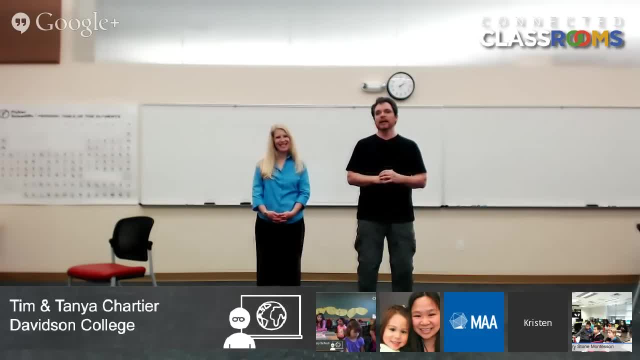 think of, but that's about all I have there. but there's a lot of that and actually there's a lot of what's called biomechanics in there is that when you're doing mine, if you're pushing with this arm, I make my body look like it's. 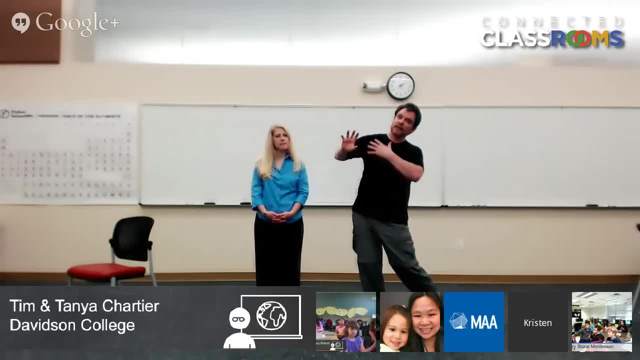 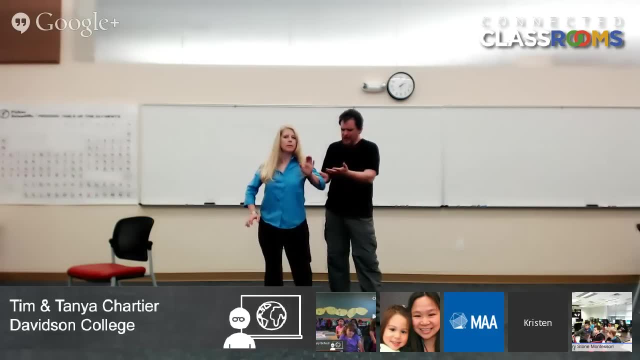 working, but I actually relax my body. I only make the part stiff that I have to. I absolutely have to. Marcel would come up on certain parts and go: why are you so? why are you trying so hard here? it doesn't need to be like this. relax, then you can perform for an hour. like this, you perform for five minutes. 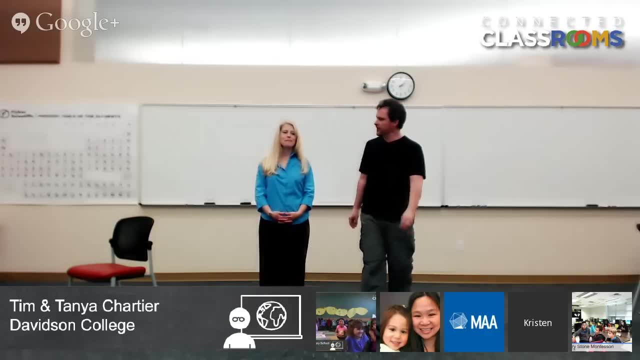 so that's probably it too. those are the ones I think of trying to make it really real, like in the physical world, and the same kind of thing in terms of our time. I think of it in terms of approximating things, thinking about the slope, the angle. that's the mathematical side of it, but I think, to make it true to life you.